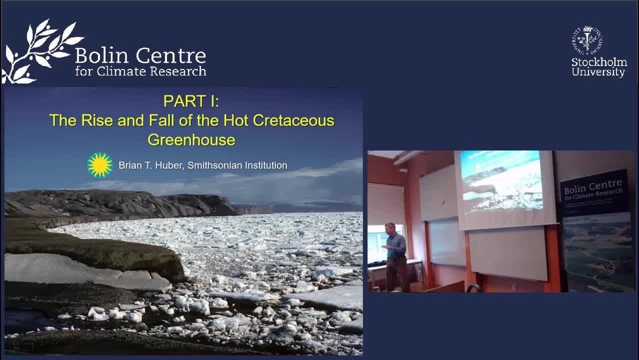 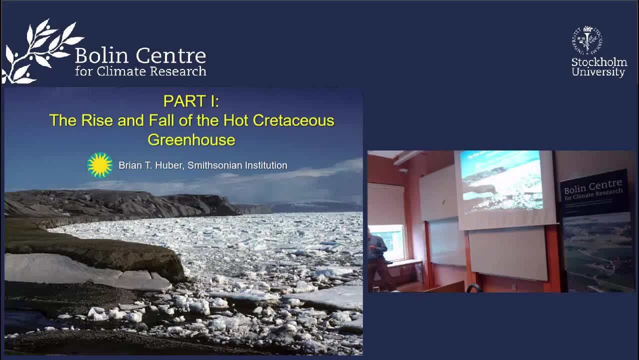 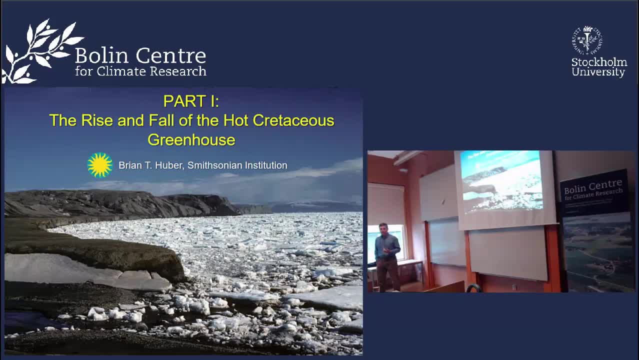 And so I'll go into how we constructed that climate curve and then the implications of that. The second part will talk about an ocean drilling expedition on which I participated one year ago, And the reason it's relevant to this talk is because I'm a member of the Cretaceous Age. 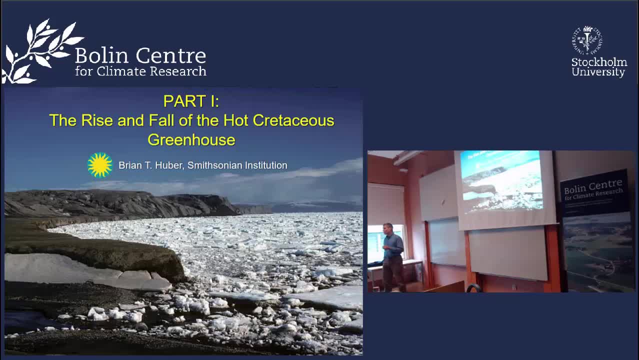 And it's a big part of this, And this is a great opportunity to push up on climate change And a lot of it is based on the climate change that's happening in the Pacific and the perspectives of the island and the climate change that's happening in the Pacific. And the reason I have it so important is because the purpose for that expedition was to fill in gaps for the climate curve, And so if after the first part you feel like you're done, I won't feel offended if you want to get up and leave. 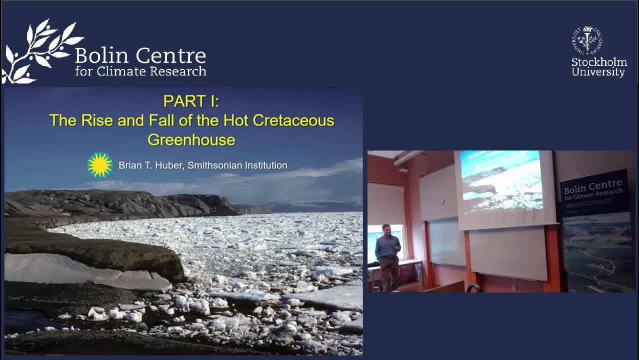 But actually the two talks it should go together pretty well. I start with this slide because I think it's a really neat, interesting juxtaposition of modern day icehouse climate and the climate change that's happening around us, And in this case it's a really interesting juxtaposition. 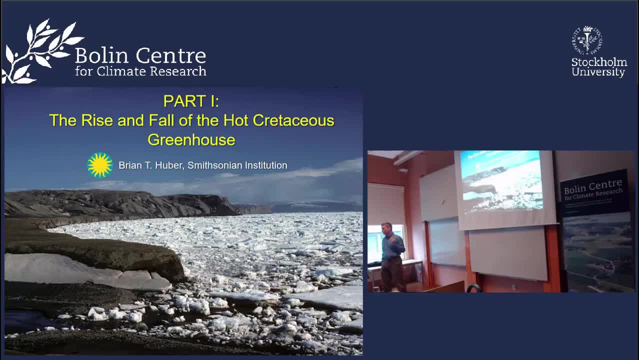 Antarctica. in Seymour Island, which is in the northeast Antarctic Peninsula, The Cretaceous sediments are in the background and this is where I did my master's thesis work. These sediments dip eight degrees to the east. We've got a record from the west end of the island that goes up through the Cretaceous 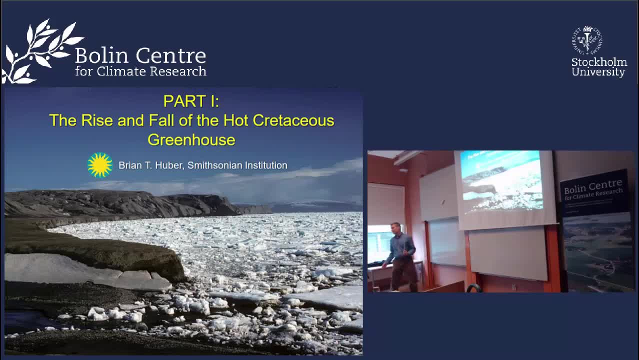 Palaeogene boundary from about 74 million years up to about 55 million years ago, going this direction. So I was a young graduate student when I went there camping in tents for three field seasons, collecting through the sequence and the thing that really struck me: how do we advance? actually, how do we advance? 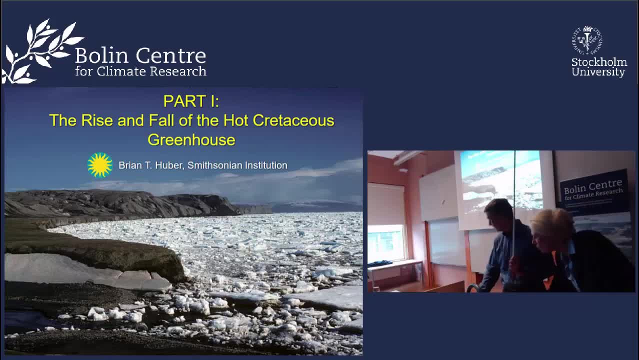 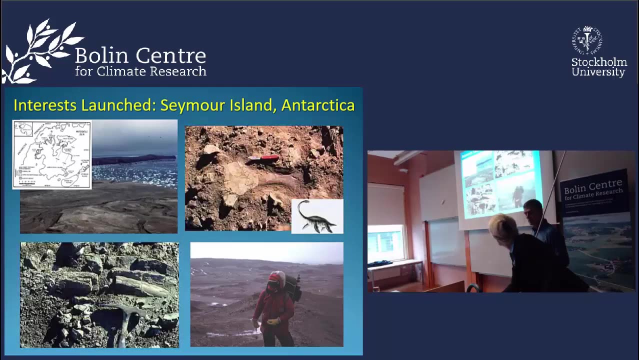 the page. So just hit this, okay, yeah, okay, very good. So the location where we worked is Seymour Island, here with the Cretaceous sediments on it. It's in the Antarctic Peninsula here, 65 degrees south and just as. 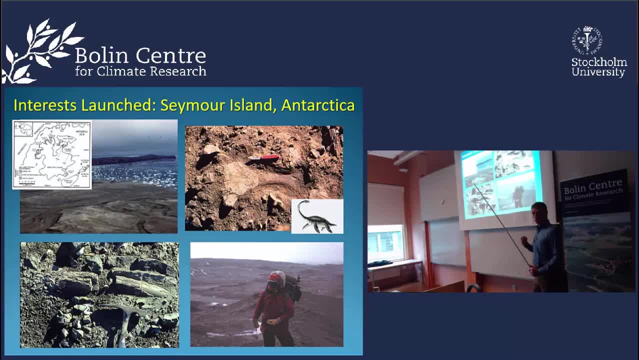 an aside, this is a location where the Nordenskold expedition visited in 1901 to 1903.. The Swedish North Polar Expedition built their hut right here and they spent most their time collecting from Seymour Island, and they went there because whalers brought back fossil wood and ammonites, evidence of a very 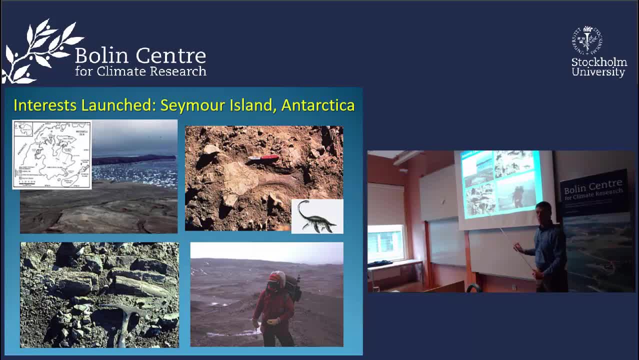 different earth and there was interest to find out more about this location. So for two years the Nordenskold expedition was here. they collected from Seymour Island and the fact that we found fossil wood in Antarctica was quite dramatic at the time of this expedition and of 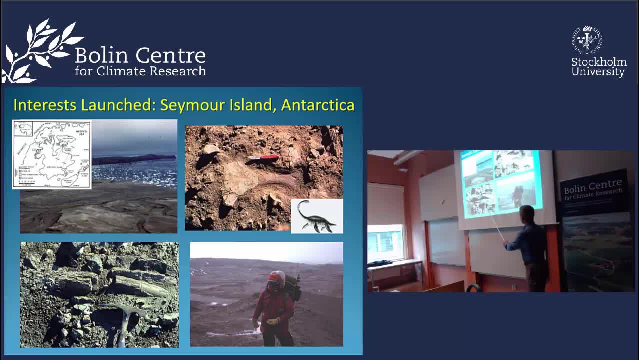 course, when you're working there and it's very, very cold and you see fossil wood and you find plesiosaur bones, which is an extinct swimming reptile, cold-blooded, it tells you it was a much warmer climate. So from the beginning of my research, I've always had a deep interest in 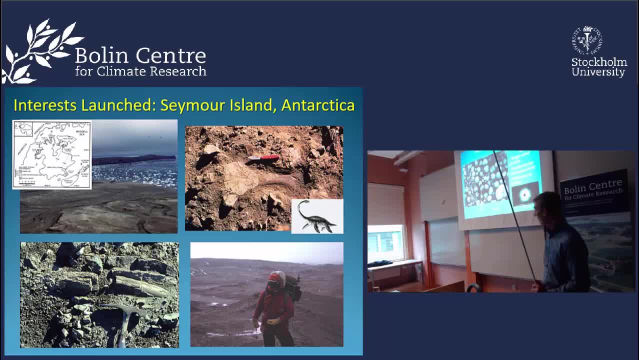 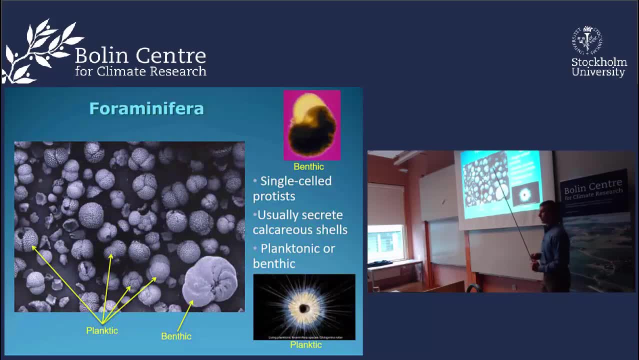 understanding Cretaceous climate. As Helen mentioned, the focus of my talk will be about foraminifera, and these are single-celled organisms that make a shell. There's two kinds benthic lives in the seafloor: planktics- floated. They're in. 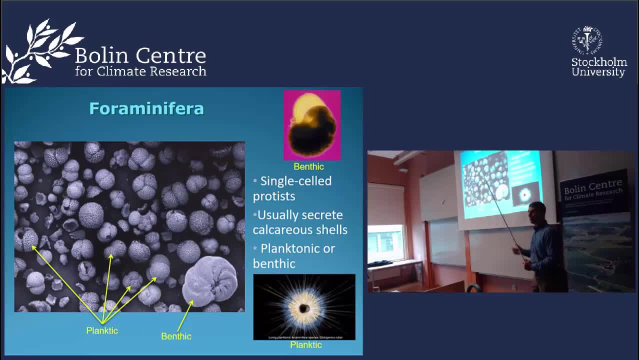 the ocean today and they have a fossil record going back into the Jurassic. in fact, for the planktics, This is a slide of Eocene foraminifera with many planktics foraminifera and one benthic foraminifera, and so these are the 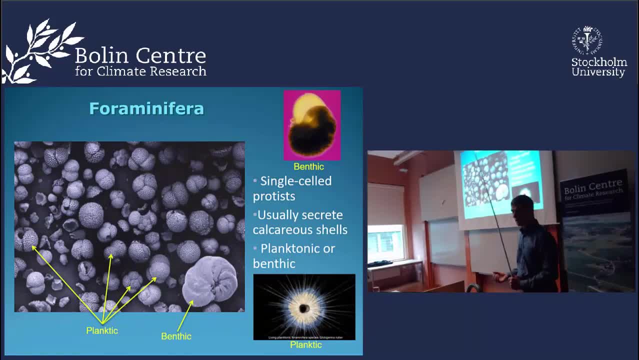 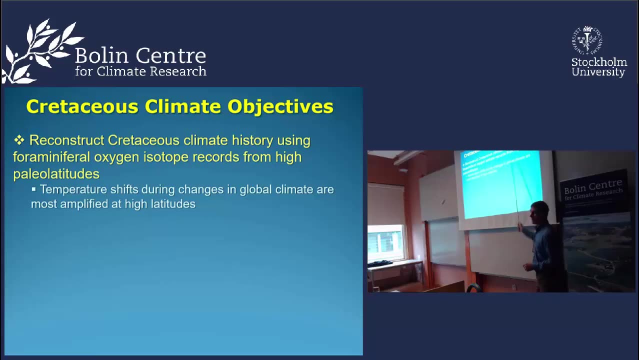 shells that accumulate that are very useful for telling geologic age, but also, as Helen mentioned, chemical analysis of the shells allows reconstruction of temperatures. So the goals for this part of the talk is to reconstruct the Cretaceous climate history. So the first part of the talk is to reconstruct the Cretaceous climate history. 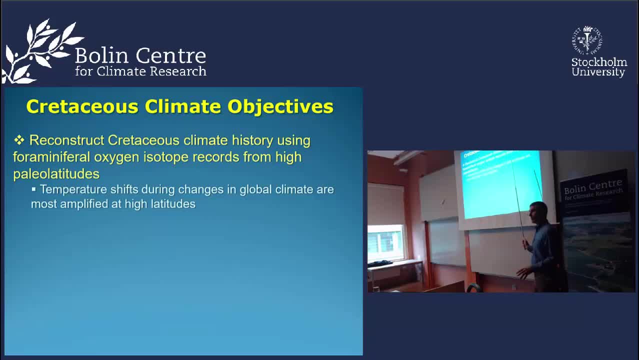 From high paleolatitudes- by high, I mean on the order of 60-62 degrees south paleolatitude- And so we want to look at how the temperatures changed. what were the maximum temperatures? and then at what time did temperatures warm versus? 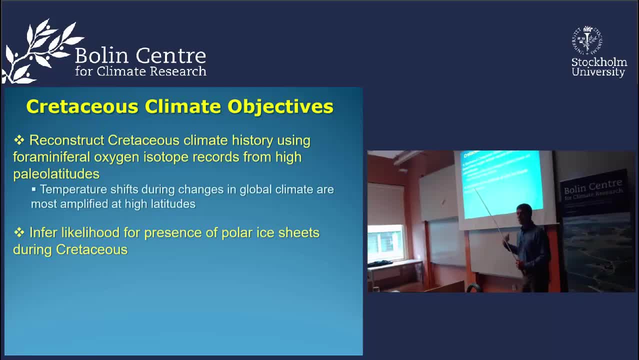 cool. Based on this, from the high latitudes, we are interested in whether or not it was cool enough to support continental ice sheets in Antarctica In, In particular, there are Cretaceous sea level curves that many people have said in the past. 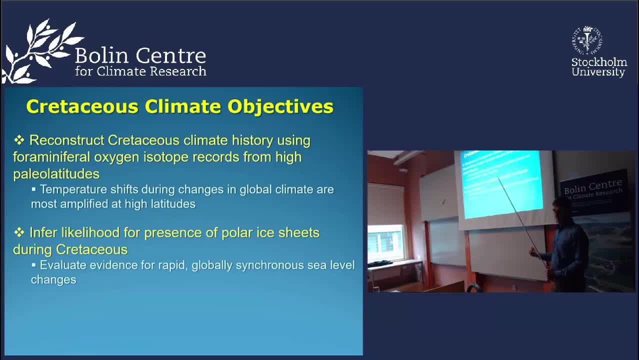 must be caused. the sea level changes must have been caused by ice, icy growth and decay. So the question is: did those ice sheets exist to cause sea level changes? And then we want to understand: okay, if climate changed, what were the forcing mechanisms? 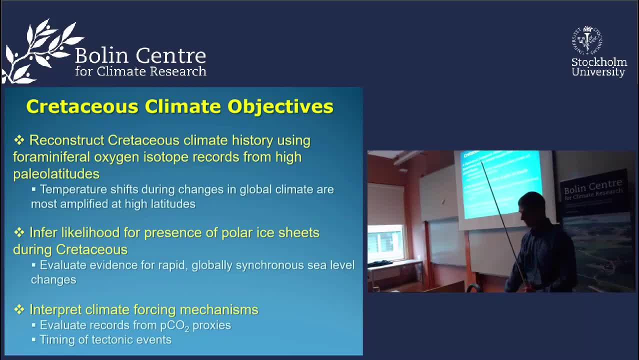 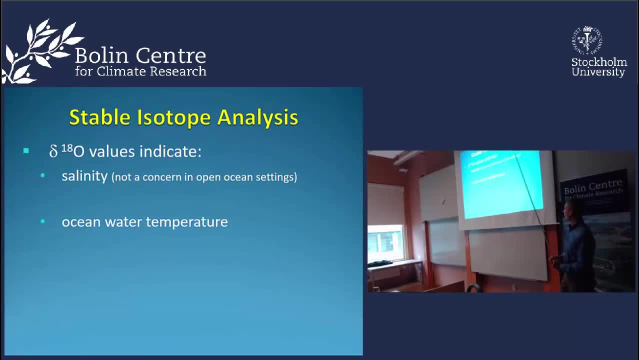 for those changed What drove Cretaceous climate shifts. So we'll talk about stable isotopes, and this is the chemistry of the shells of the foraminifera, and we will express this in the delO18 values and the oxygen isotopes. 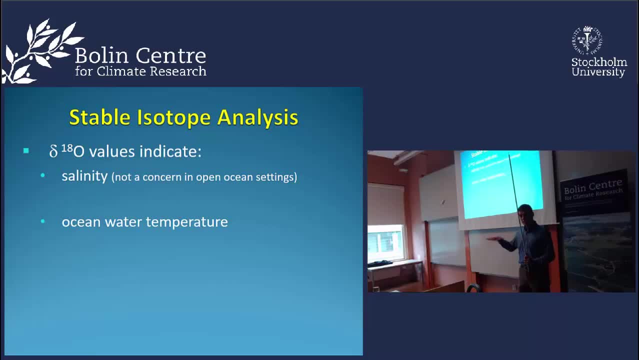 are affected by salinity, but in the open ocean salinity stays the same, so we don't have to worry about ocean salinity because we assume it's constant. Mostly the signal tells us water temperature and as oxygen isotope values become more. 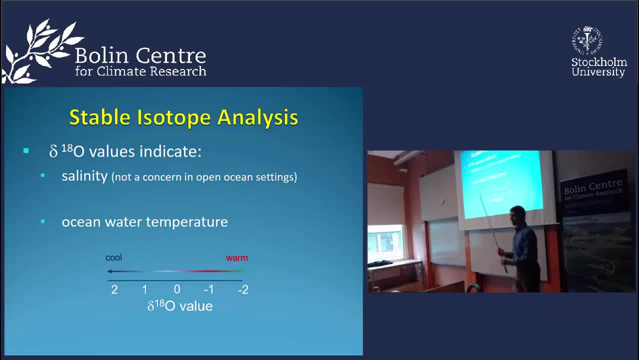 negative, that indicates warming. as they become more positive, it indicates cooling. And, of course, the planktic foraminifera which float at the surface, give you the warmer temperatures. the benthics give you the bottom water temperatures. 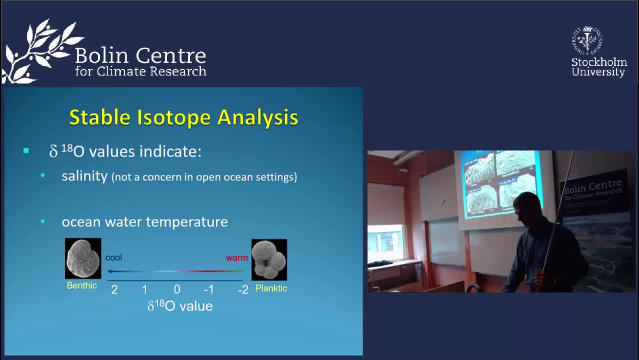 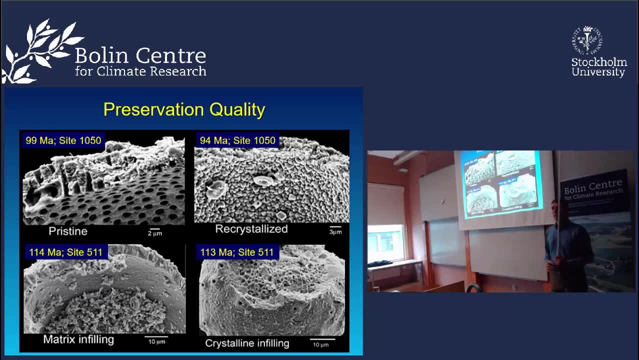 So this is a very powerful tool for reconstructing ancient climate. As we go back further in time, we have to be concerned about preservation of the shells. The ideal preservation is this Very pristine shell wall with the pores perfectly preserved, nice layering of the shell. 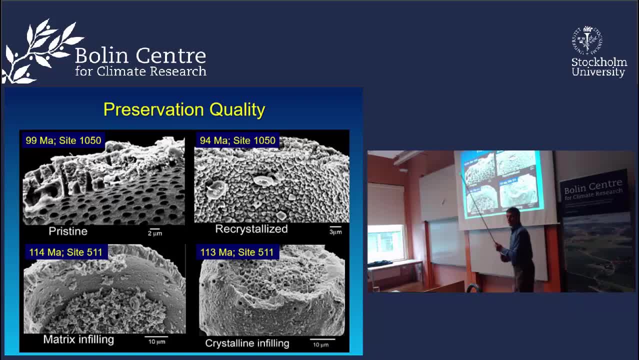 This particular shell is actually 99 million years old, yet it's still perfectly preserved because it was deposited in clay-rich sediment. This shell shows re-crystallization, which means the pore water has slightly changed the chemistry of the shell, so oxygen isotopes from a shell like that are going to be a little. 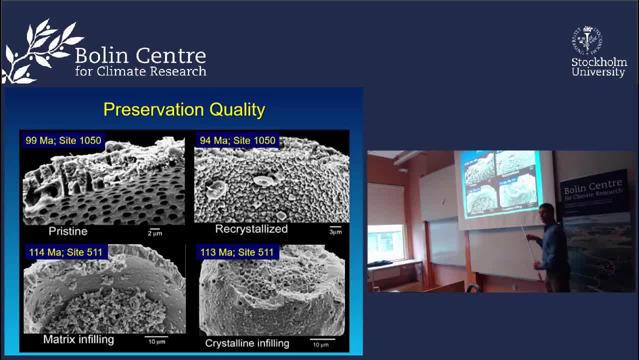 bit changed. This shell is completely filled in with calcium carbonate, And that calcium carbonate completely changes the signal, and so you can't really trust a signal that's infilled like this. This shell is just dirty. The shell itself is okay, but it's just infilled with matrix. so you clean your forearms and 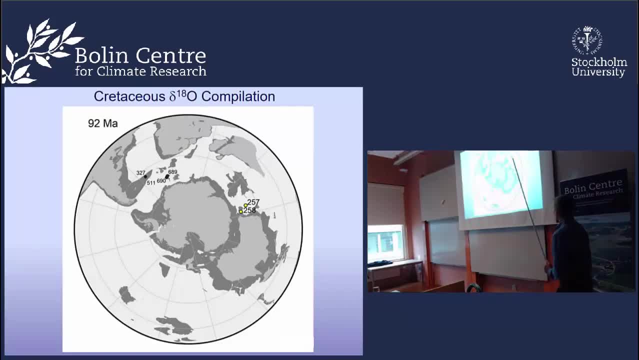 then you get a fine signal. The locations that I'll talk about, where we're getting our temperature curves, are shown in this map, Reconstructed for 92 million years ago. The temperature curves are shown on this map, reconstructed for 92 million years ago. 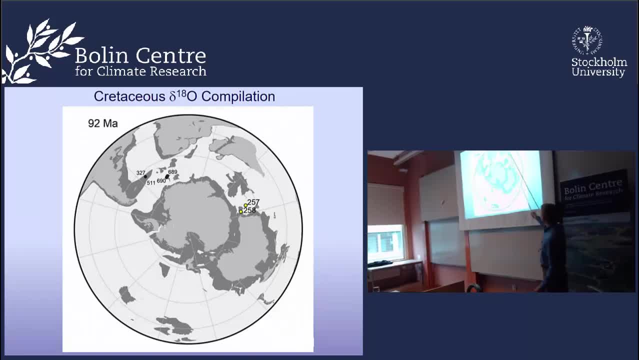 Australia is up against Antarctica, India is in the southern Indian Ocean, here is Kerguelen Plateau, and then South America and Africa are closer to Antarctica as well. So all these sites were around 60-62 degrees south. In particular, I'm 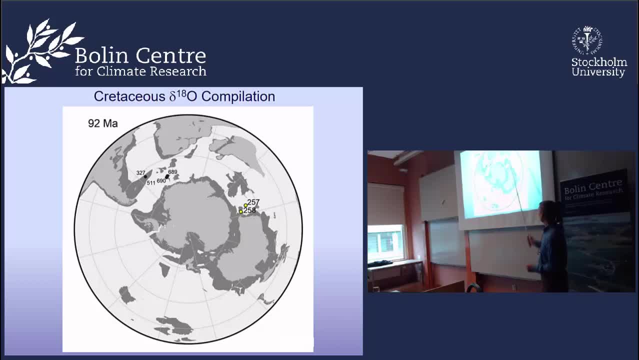 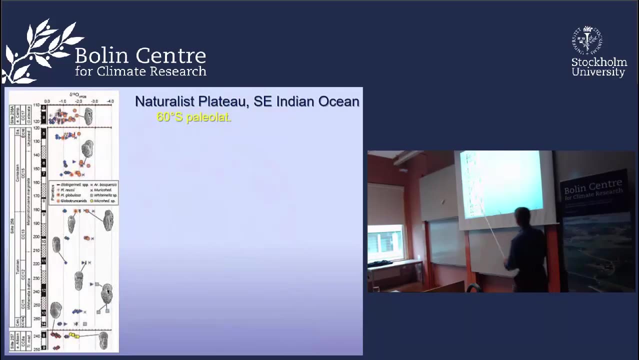 going to focus on these two sites in the southeast Indian Ocean. These sites were drilled in 1972 by deep-sea drilling project and the drilling was incomplete, so the record was incomplete. This shows the Cretaceous record. The black represents sediment that was recovered from the coring from the drill. 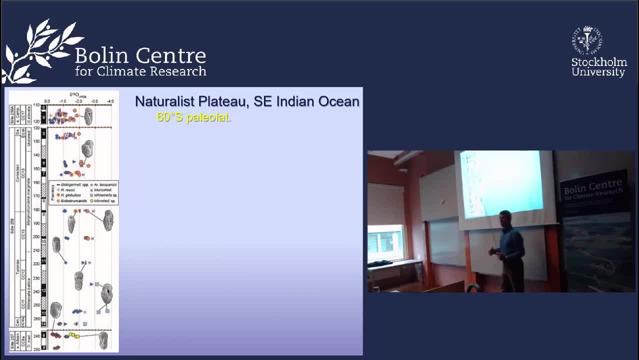 ship. The white and the diamond pattern represents unrecovered intervals, So we have very brief intervals where we can get data. Nonetheless, my colleague Ken McLeod and I analyzed the benthics shown as diamonds and the planktics shown as the circles and the crosses and triangles Starting in the 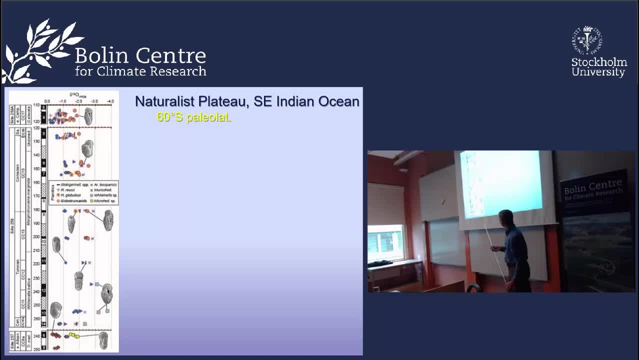 late Albion, which is on the order of 100 million years ago. our benthic temperatures are shown here. planktics: here We see that they're pretty consistent until we get to the Toronian, which is this age here where we get. 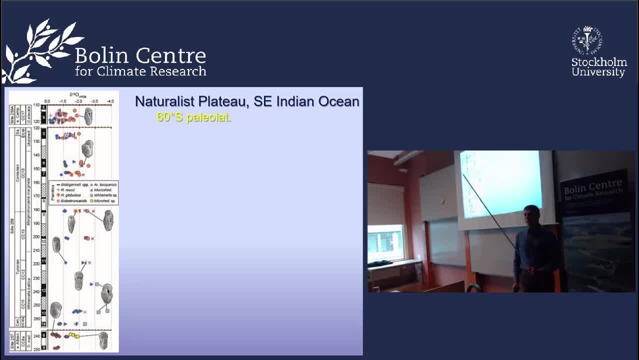 values of minus 3.5 per mil And when you reconstruct the temperature of those values at 60 degrees south, the temperature would be on the order of 30 degrees centigrade at 60 degrees south. So the benthic temperatures- here you can see they shift to warming, here increased to. 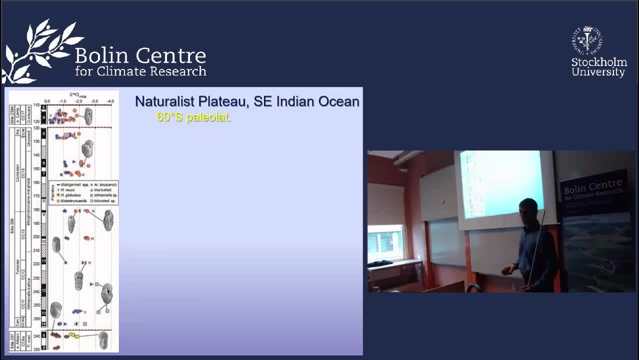 18 to 20 degrees centigrade in middle baffle depths. So we're going from a warm climate to an extremely hot climate. But you can see there's lots of gaps in the record, so there's details that are not in this record. Nonetheless, it's these: 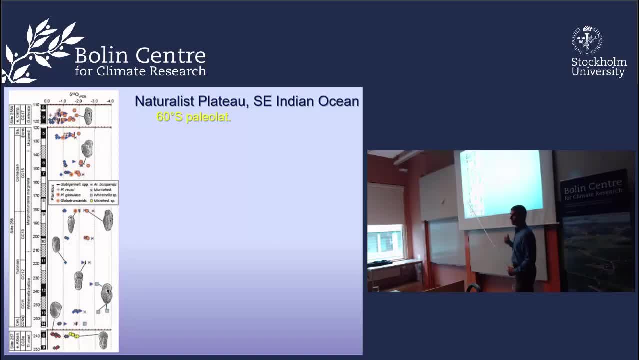 data that were the basis for constructing a proposal for ocean drilling to fill in these gaps, and I'll talk about that in the second part of the talk. Notice that the temperatures stay very warm and then they start to cool up here and become more positive, which means cooling, Preservation of the 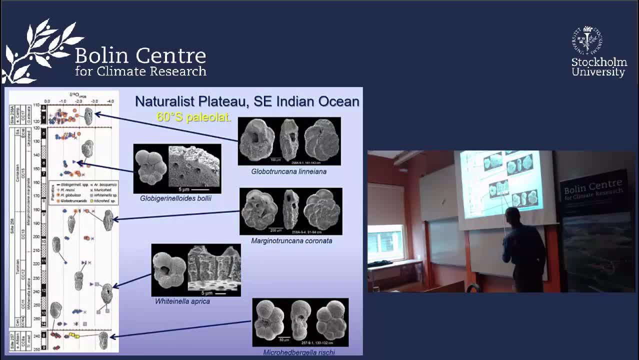 foraminifera is really nice all the way through, and so you can see beautiful shell preservation here, nice shell preservation here, and so these are reliable data from the southern Indian Ocean. And what I did with those temperatures. I went back and looked at them and I found that they were pretty. 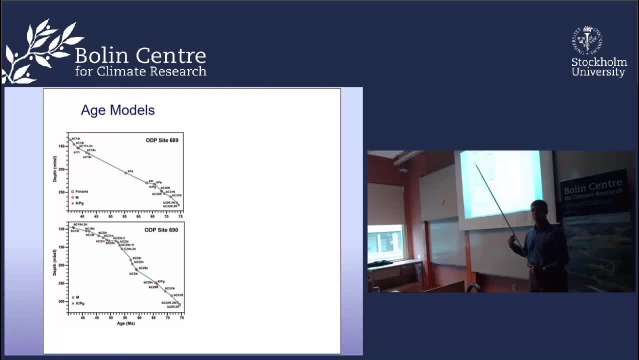 good. So I went back to all the sites where we've gotten oxygen isotope data- from the southern South Atlantic as well- and reconstruct new age models to provide age constraints for all the data that have been published in the past, particularly data I've published but also colleagues have published. So this 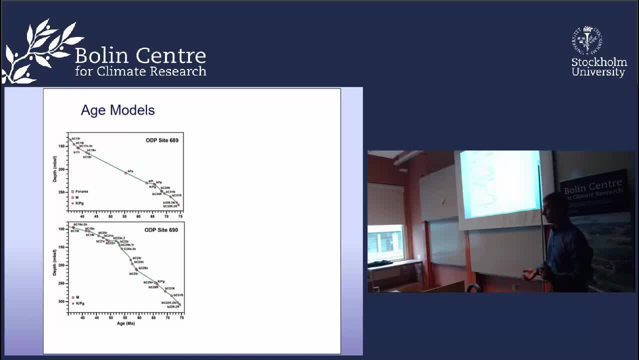 is the age depth curve using a combination of calcareous nanofossils, foraminifera and paleomagnetics. So what I'm showing these graphs is that we actually have quite well resolved age determinations for all these different sites, which means every core sample. we 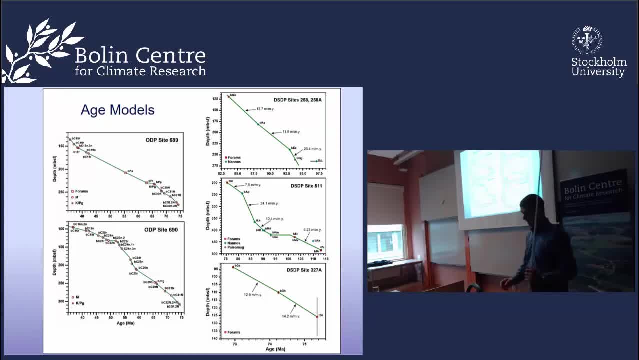 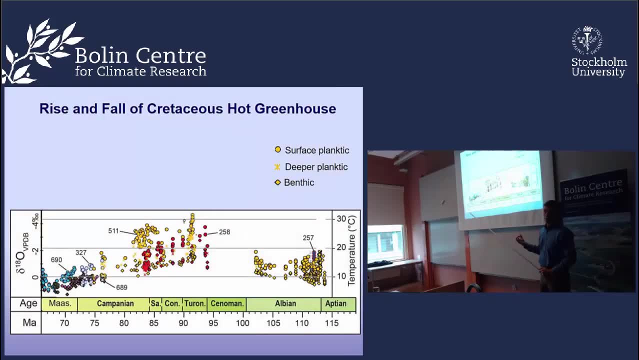 get, we can get a pretty reliable age for those samples. So once we've done that, then I've plotted all the data on a common curve, for the southern Indian Ocean, shown in red, and then the southern South Atlantic, shown in the orange. 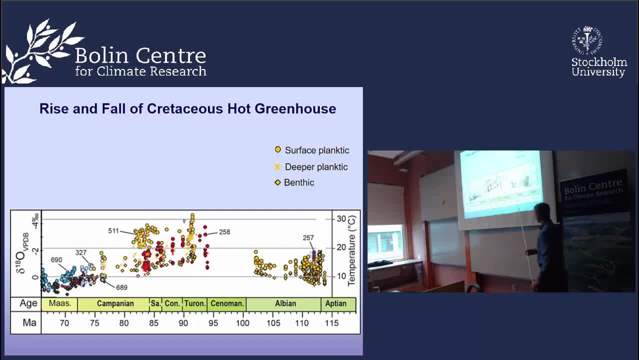 and these colors here. So again, if we start back at the older part of the curve, this is 114 million years ago, where the data start. we've got the benthic data, which are diamonds, and these are the temperatures here: 10 degrees C So it's. 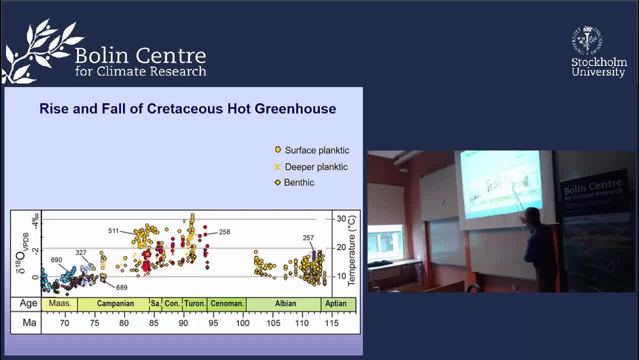 warm relative to today and you see slight warming as we get into about 104 million years ago. And then we've got a big gap with no data because of the drilling. recovery was not good. Notice we've got this abrupt shift. 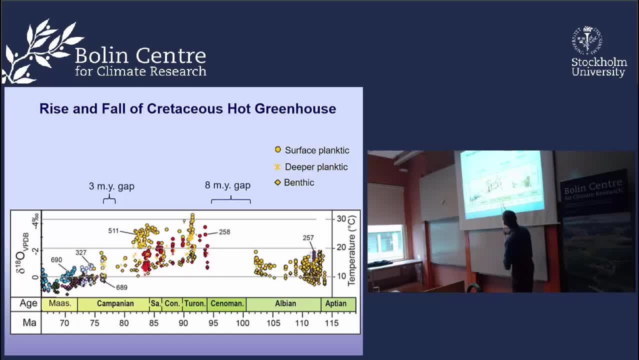 from the warm temperatures to really hot temperatures right here, Right across the Cinnamane-Eutronian boundary at about 94 million years ago. So a big shift here. And then notice the Atlantic data stay warm, the Indian Ocean data start to cool. 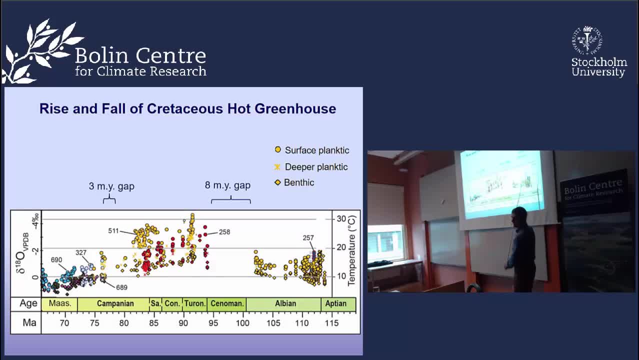 But the warmest values are more than 30 degrees centigrade. Again, to remind you, this is at 60 to 62 degrees south, with temperatures this warm Also at this time, this is when we've got dinosaurs in Antarctica and fossil forests. 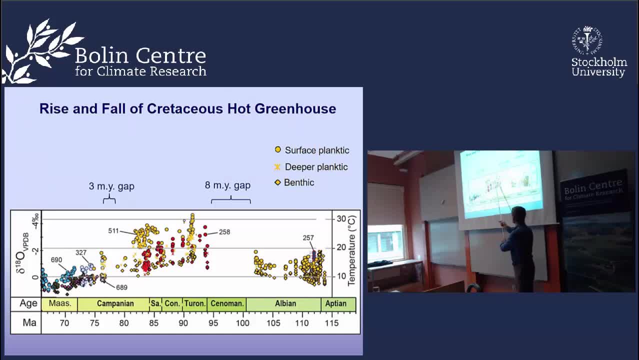 So we know from the fossils that it was warm. This is telling us it was almost tropical. So it's kind of alarming because climate models cannot model these kind of warm temperatures. So the big question is: how abrupt was this shift? Did it happen very quickly? 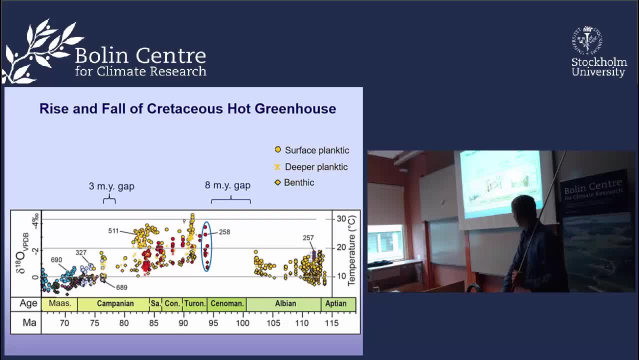 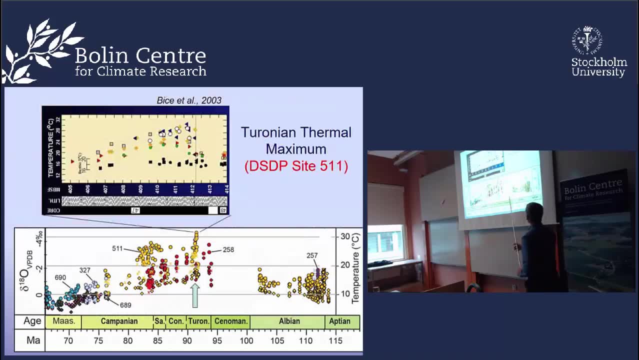 And was it because of volcanism? But what caused that temperature warming? We have that big data gap and so we need context for that warming. Work with Karen Bice back published in 2003,. we looked at southern South Atlantic data site 511,. 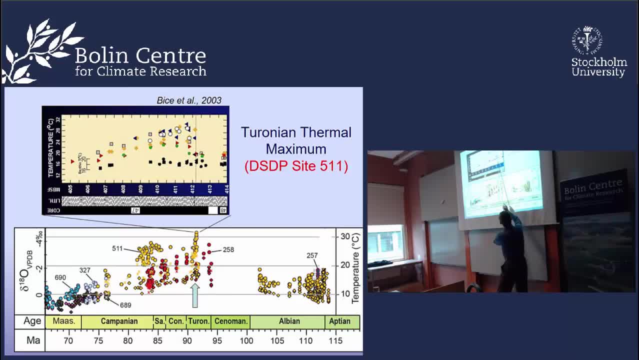 Falkland Plateau And we took apart the warming event with the different planktic species up here. These are the benthic species And we see that it's a surface water warming in the South Atlantic. Again, look at how warm these temperatures are. 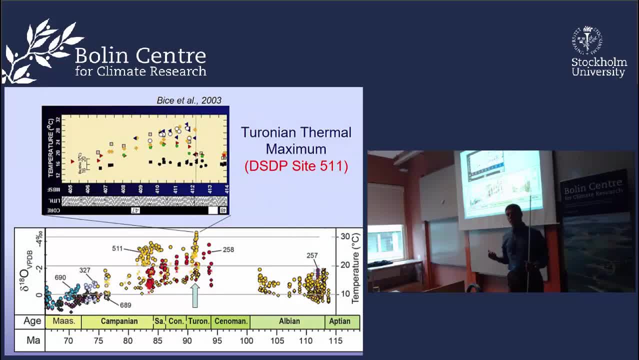 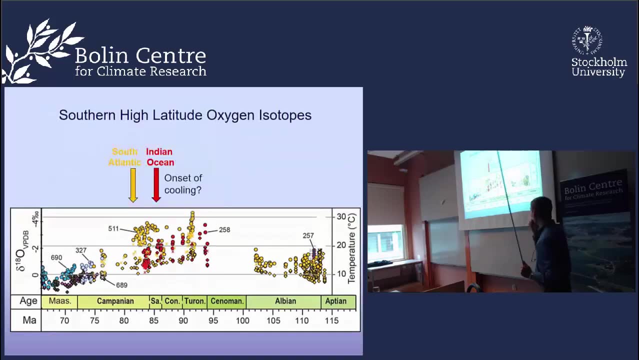 Very abruptly getting extremely warm. So we've got data from both oceans in the southern Indian Ocean and the southern South Atlantic, telling the same story that the Tronean age, which is right here: It gets extremely warm. It's interesting that the timing of the cooling 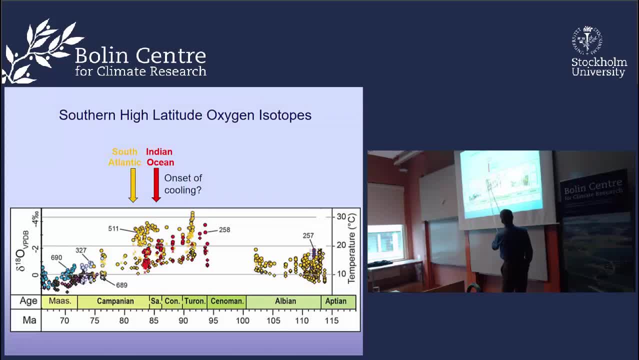 is different between the Indian Ocean and the South Atlantic, So it seems like the South Atlantic stays warm longer than what happens in the Indian Ocean. So we're going to test this with the additional samples that we've poured. Then notice we go from temperatures that are really 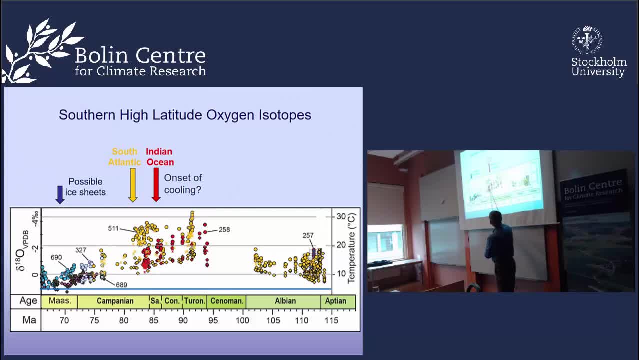 warm The big difference between the planktic temperatures and the benthic temperatures. And then the planktic and benthic temperatures converge as we get into the younger sediment at about 70 million years ago. So there's very little difference between the planktics. 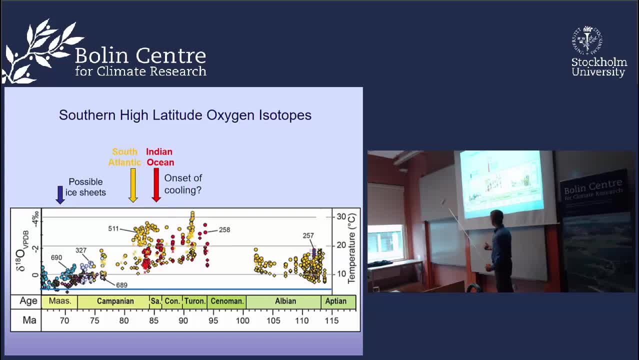 and temperatures, which means a very mixed ocean and a much cooler ocean, And it's almost getting to the point where the temperatures are cool enough for at least small ice sheets in Antarctica. And then notice, at the end of the Cretaceous we have a very 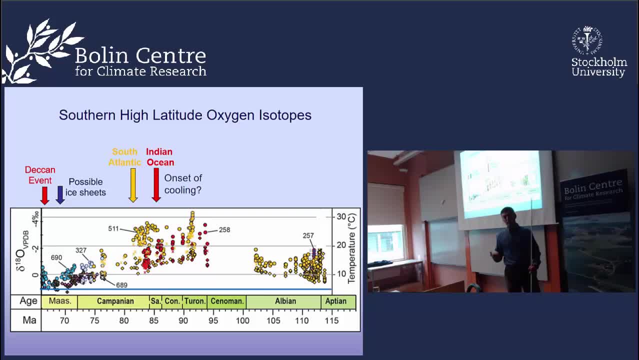 very brief warming event, And this is when there is a big volcanic eruptions series in India called the Deccan volcanism event. And so this Deccan volcanism is pumping CO2 into the atmosphere and causing global warming, And you can see that quite nicely represented. 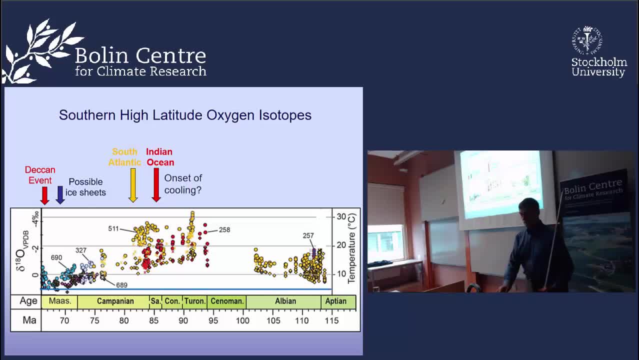 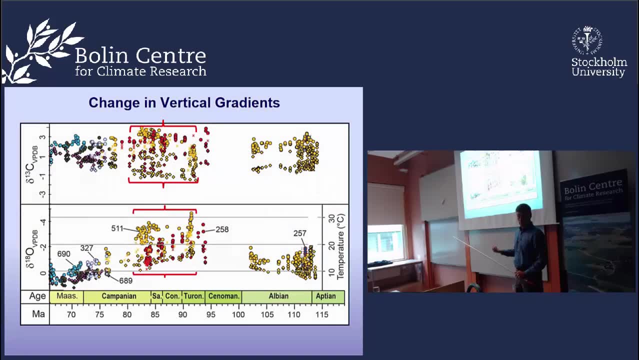 the last 300,000 years of the Cretaceous. When we measure oxygen isotopes at the same time, we get something called carbon isotopes, And this tells us something about the carbon budget in the ocean And the difference between planktic and benthic carbon. 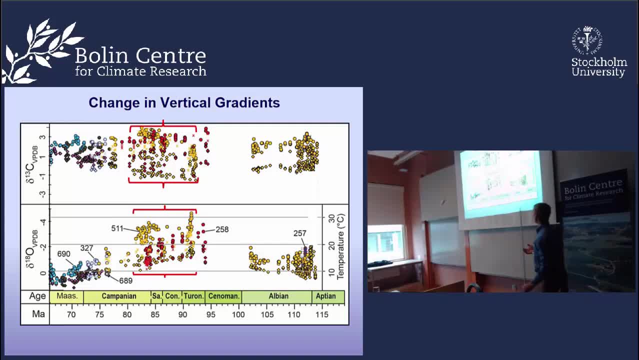 isotopes also has something to do with productivity And it basically is a paleo oceanographic tool. What's interesting is we have very high gradients between the surface water and the bottom water for both carbon isotopes and oxygen isotopes, which suggest a very layered ocean at this time. 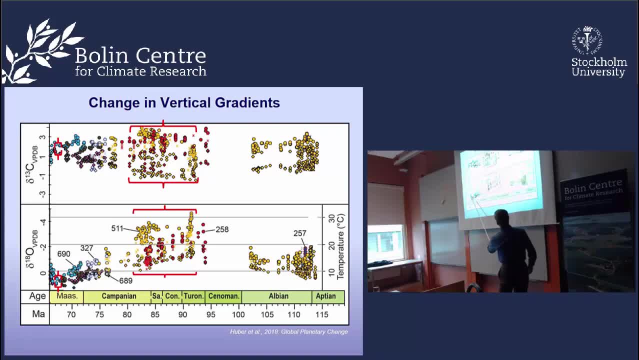 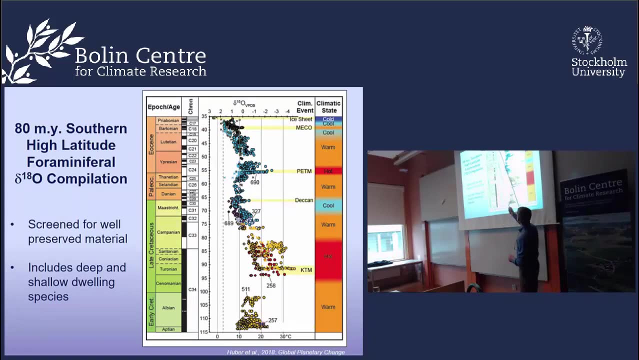 OK, And again contrast that with the very small gradients we have toward the end of the Cretaceous, which suggests a very mixed ocean. So this is a long-term curve from 114 million years ago to 35 million years ago, And Helen and I call this the PETM Smackdown curve. 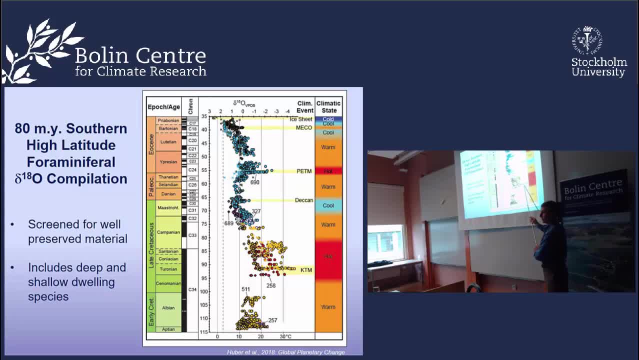 Because if you look at the temperatures achieved during the Cretaceous thermal maximum, they're actually much warmer than anything you get at the PETM at high latitudes. Even for the benthics, we are on the order of 20 degrees C. 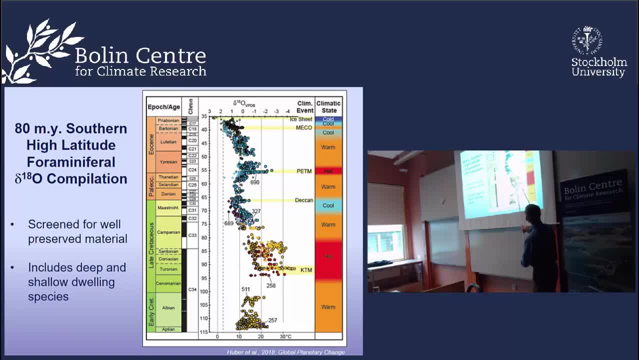 with the warmest temperatures here, 24 degrees C. So in terms of a mechanism for warming, we seem to have a much hotter greenhouse Earth throughout this whole interval from Tronion through Santonion relative to anything that occurs. So we've got a hot greenhouse throughout this whole time. 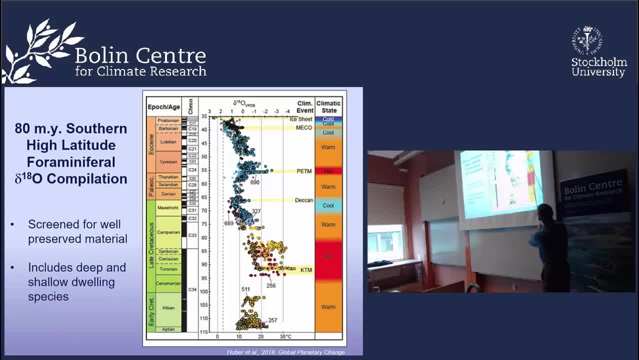 and then gradual cooling, And then it warms up to the PETM, which is a brief hot interval during the early Eocene, And then you see gradual cooling And then ice sheets form. in Antarctica. A continental ice sheet forms right at about 38 million years. 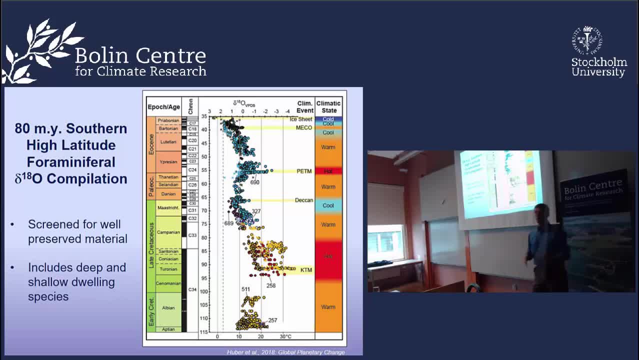 ago, And this is when we get a very large ice sheet reaching sea. This is a very large ice sheet reaching sea level in Antarctica. This is sort of the Delo-18 value, where ice sheets form very large continental ice sheets where the temperatures are cool enough for large ice sheets. 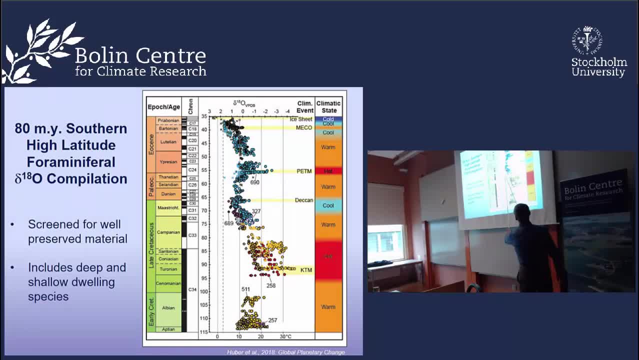 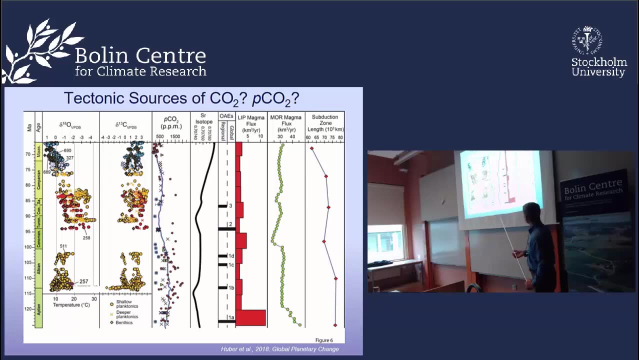 And you can see the Cretaceous temperatures never really get down that cool. We get close right here, but it never gets cool enough to form a large ice sheet. So I wanted to. I've asked the question: how do the proxies for CO2? 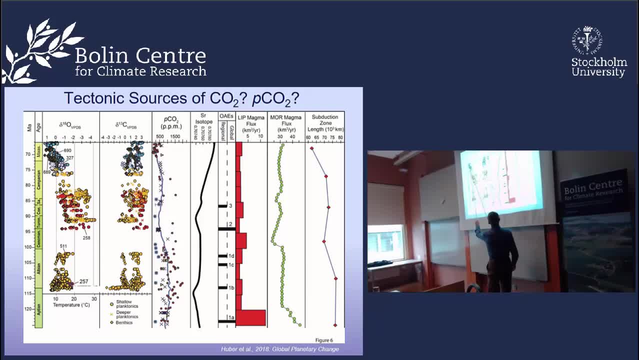 compare with the temperature curve shown here, And we have multiple proxies for estimating carbon dioxide from the Cretaceous And one is from leaf stomata, And this is what Margaret does here and a colleague at the Smithsonian is working on this And a number of people measuring the stomata. 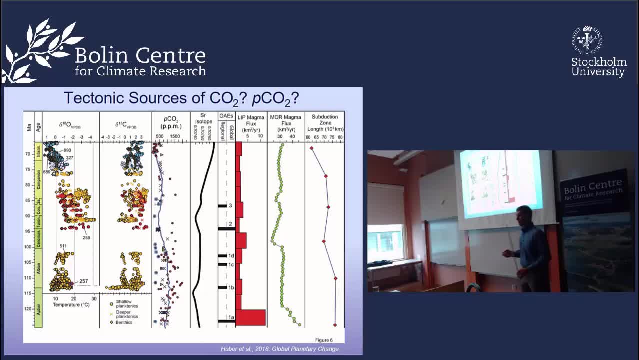 from the Cretaceous And the problem is that if the CO2 is being generated from the Cretaceous, then we have very low leaf stomata index values And we can see that from particular leaves, that the density of the stomata is relative to the carbon. 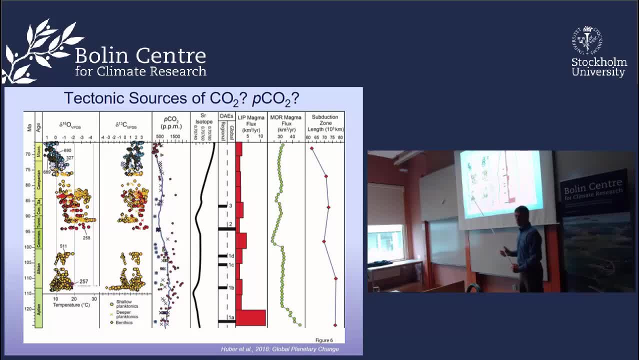 dioxide. The problem is when we have the warmest temperatures. here we've got very low leaf stomata index values for the Cretaceous, So there's not good correlation for that. Another approach for estimating CO2 is from paleozole. 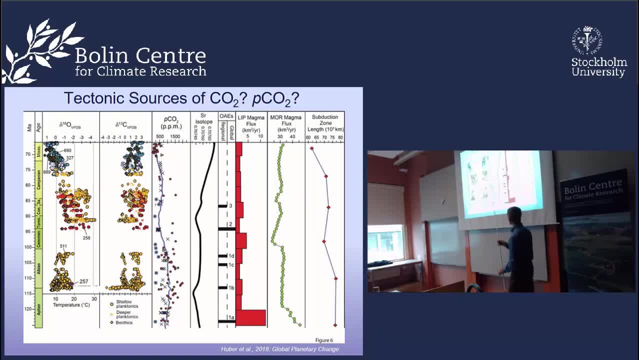 and measuring the carbon isotopes from the paleo souls. and again the peak of the tronion. it really doesn't stand out. there's not much data. these circles here, not much data. so there's not good correlation from our pco2 proxies. the other driver for temperature is tectonics, and so the large igneous. 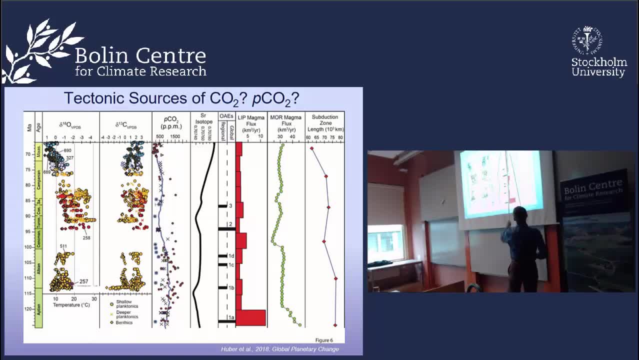 province eruptions. this that's what LIP stands for. so magma flux: there's no big peak that corresponds with the peak temperatures here. mid-ocean ridge magma output: also no big peak corresponds. and then the length of subduction zones. when you plot that in a curve, again there's nothing that stands out that strong. 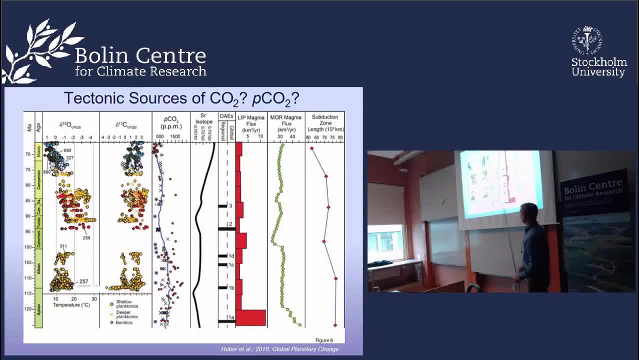 shows a strong connection or correlation to dry, extremely hot climate here. so there's there's difficulties with the proxies, so diagenesis is one. the leaf stomata: the age resolution is not great where the leaf stomata samples have been obtained and there's uncertainty about the proxies. 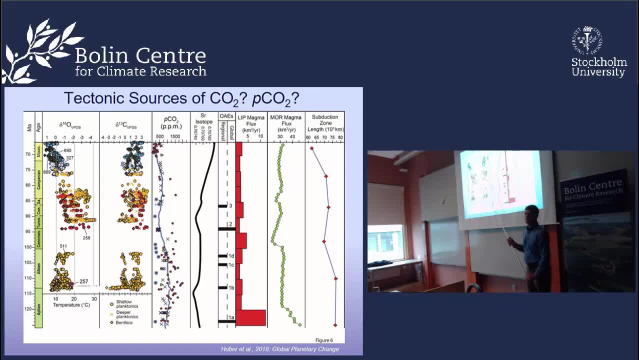 itself and, of course, for the tectonics. with with subduction, a lot of our record has been subducted, and so we may be missing some of the large igneous province eruptions that took place, and so, because of the good preservation in both ocean basins, I think we can be say that this is a very 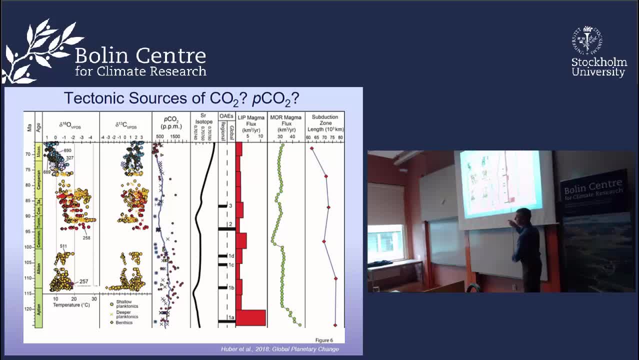 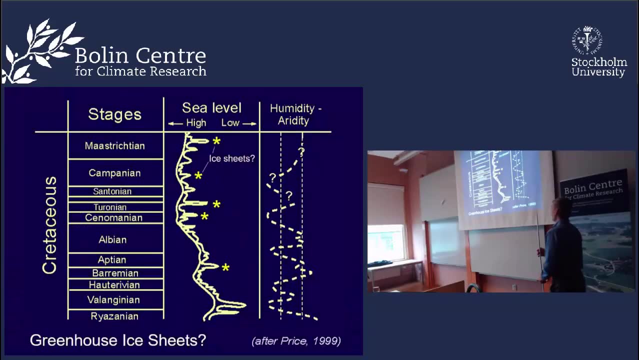 reliable signal of extreme warmth. I think the other data just need to catch up or we may not be able to find the correlation that we search for. nonetheless, this gives good reason to look you. so for the cretaceous, we have the sea level changes that have been in the 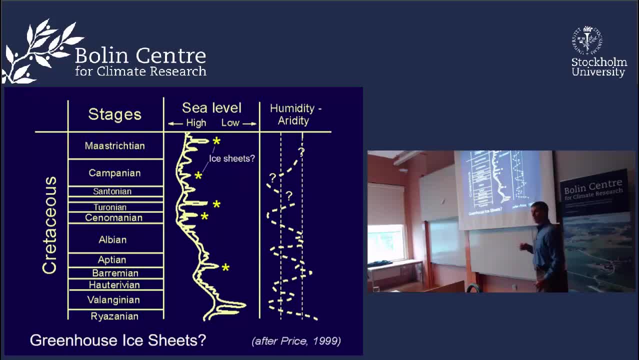 record and published that are considered third order sea level changes, which means there rapid and that there of a magnitude that they were quite large, so on the order of 50 to 100 meters sea level change in the cretaceous. so these have been estimated looking at outcrops of sections in the western interior of 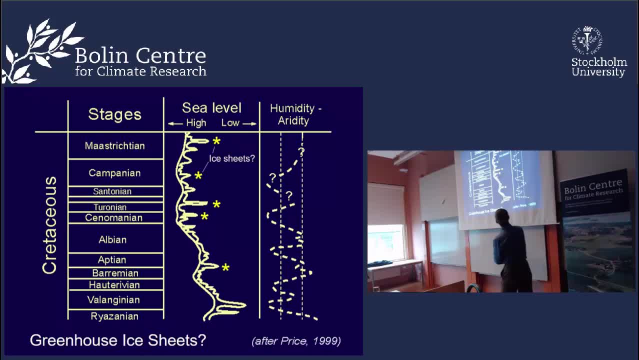 US and other locations, and this is a relative sea level curve published in 1987,- and Price suggested that there were ice sheet events at each place where there's a star, And so the question is, if we have these extremely warm climates such as this one in here, can we have ice sheets at this time? 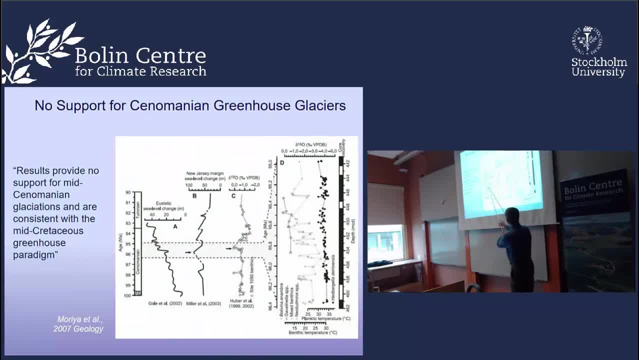 And one of the a couple of studies that suggested ice sheets during the Cinnamanian, which is this time of extreme warmth. Here's a sea level curve from Andy Gale and others suggesting a big sea level drop right here, Ken Miller. 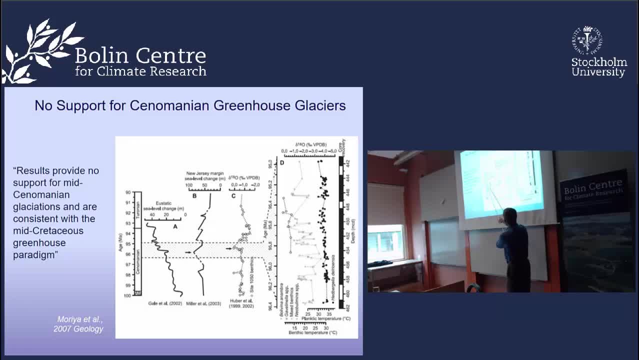 and others suggested New Jersey sea level change right here caused by ice sheets. Both of them said there must have been ice sheets in Antarctica. We published a curve of oxygen isotopes that suggested a negative shift, which Ken Miller said must be because of an ice sheet. 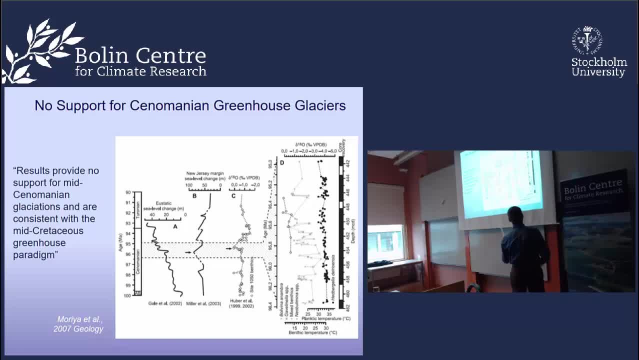 However, Mariah et al published this curve from Demer Arise based on oxygen isotopes of planktic foraminifera, showing no change in the oxygen isotope values, indicating because ice sheets store oxygen isotopes in the light isotope oxygen 16, with no change in this curve. Mariah et al said there's no way. 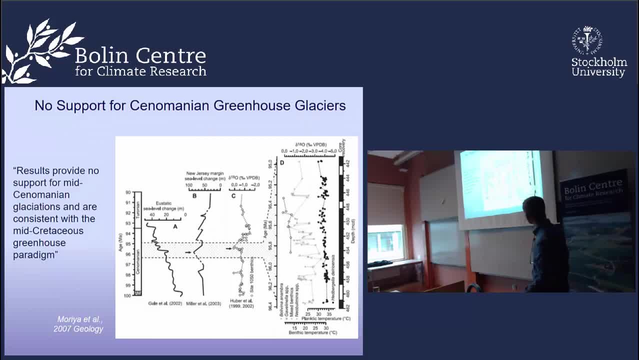 we could have an ice sheet in Antarctica during the Cinnamanian. As Sushiando and I and and a couple other authors re studied this interval. Basically we said this positive shift in oxygen isotopes is an artifact of diagenesis or change in the preservation. So we go from good preservation here to 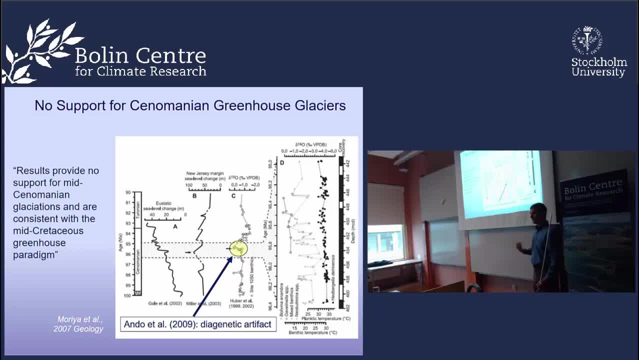 bad preservation here. So it's not a real indicator of the oxygen isotope composition of the ocean or it's not representative of that type of vertebrate bend and the situation, Remembering the ENMI, It's just not the same. we ern this equation up and, down, out, and my goal was 1, 20 times. 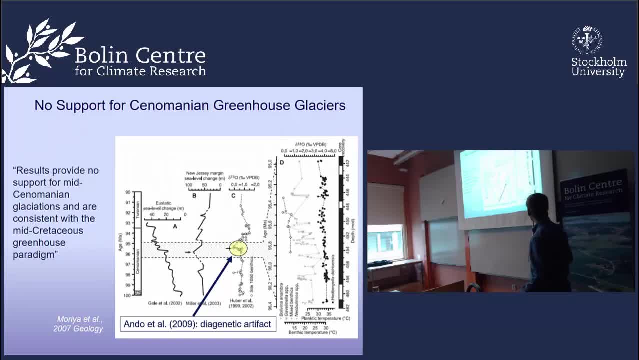 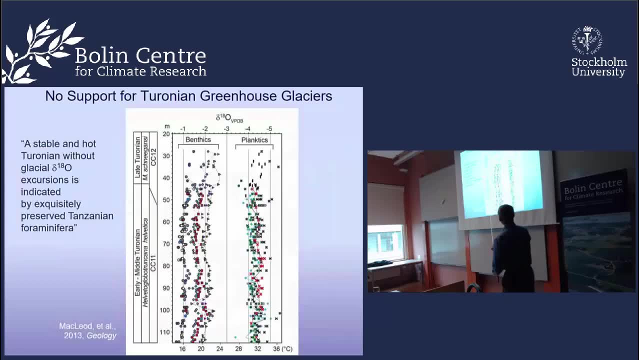 I didn't negotiate. An oxygen isotope will determine be true or proves it is. That's why there's no possibe of the level of the sodium ocean. it's an artifact, so that pretty much throws out this. the purported cinnamania nice sheet event camera cloud. myself and others published this curve. 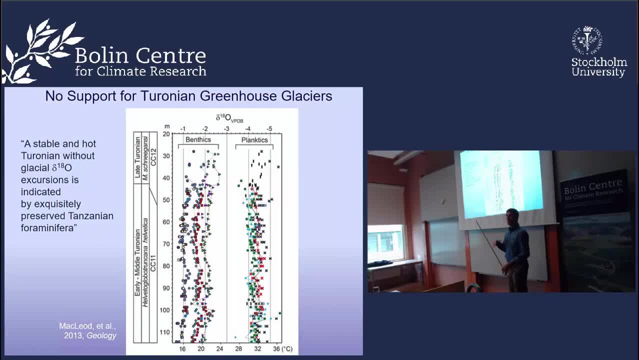 from Tanzania and this is from the tronium, which is the peak of the ice house. these are the benthic data showing different species of benthics and their action isotopes through the tronium. this is depth of the core drilled and on land, but it's all marine sediments from foraminifera and these are the plankton. 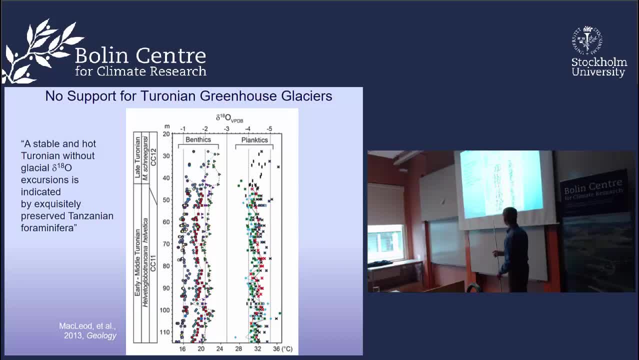 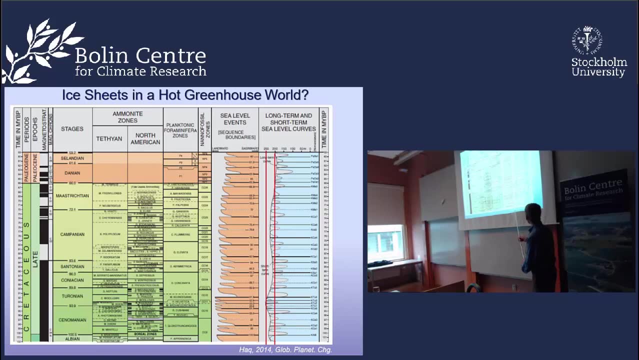 foraminifera, again, they show very consistent values and insufficient change to suggest any evidence of ice sheets. so then the question is: well, how reliable are these third-order sea level events below Hawk published a cretaceous curve in 2014, and these are the third-order events that have been. 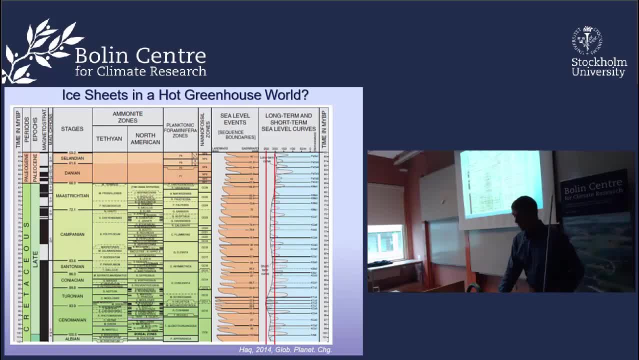 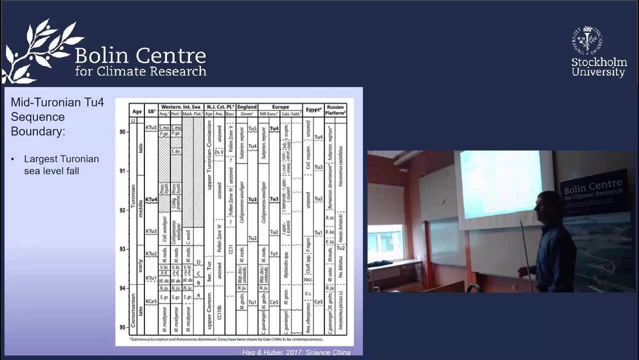 suggested to be possible ice sheet events. below is that the smithsonian now, and he and I have been working together and we focused on these two events, these two sea level events, to look at whether or not there's evidence for this change has been suggested as rapid and synchronous. 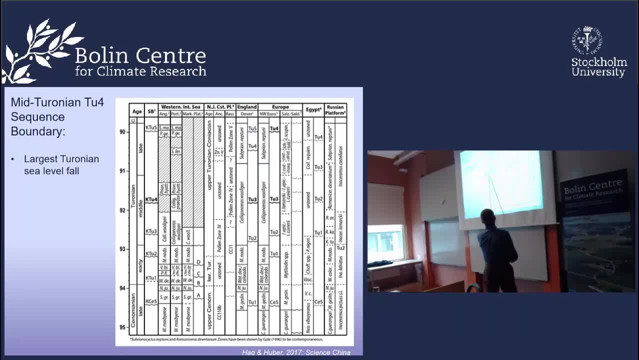 globally. so this event right here is is compared for Western Interior, New Jersey, Coastal Plain, England, Europe, Egypt, Russian platform. and the question is: is there a sea level event at all places at the same time? and basically, as we went through this, we found there were, there were. 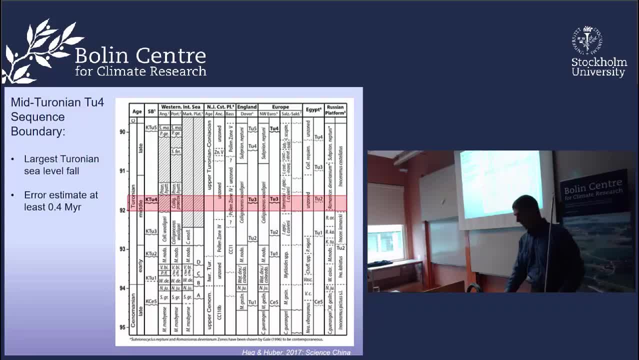 unconformities, but the basis for correlation and giving the age was very unreliable, and so the error estimates for these ages is at least point four million years and beyond that. there's no certainty that the sea level events are synchronous at all of these places, and so what blowhawk has been publishing lately is that a lot of the 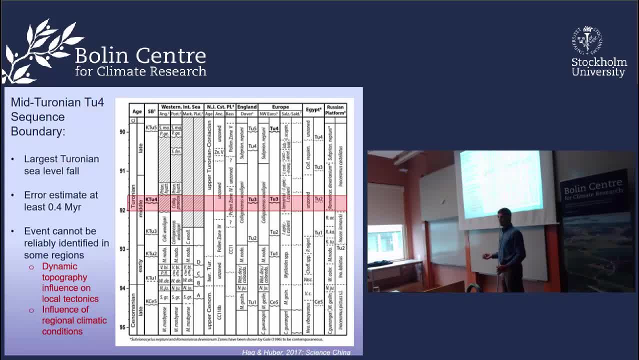 things that we thought were caused by ice are actually due to tectonics, and it's called dynamic topography, very local tectonic changes causing relative sea level change in a basin. and then the other factor is regional climatic factors, and so we are concluding that for much of the mid cretaceous to late. 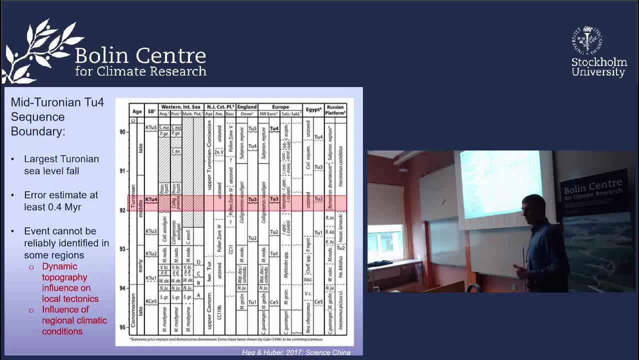 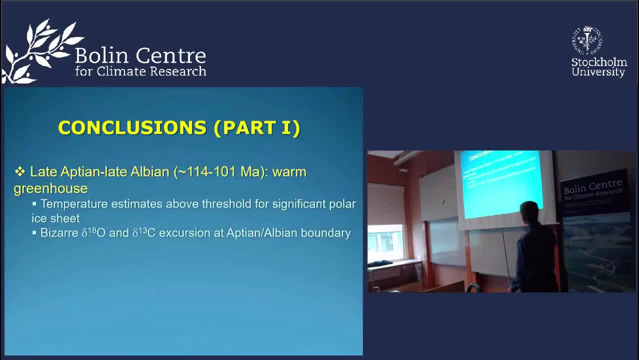 cretaceous. these so-called third-order sea level events that were considered glacial use static are caused by other factors. so I'm gonna sort of summarize this first part of the talk and this time interval. we had warm greenhouse climate throughout the earth and no evidence of ice sheets. 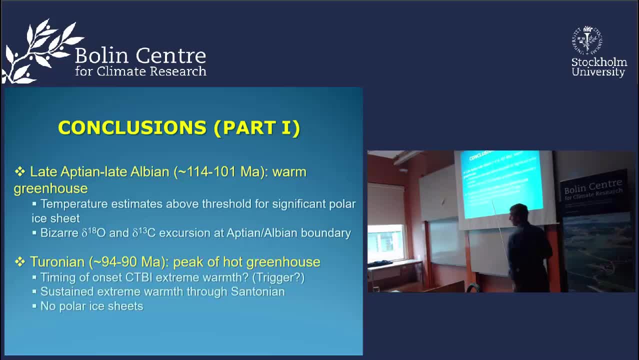 troney, we have the peak temperatures for about four million years, with extreme warmth, essentially tropical, subtropical temperatures, in the polar polar regions, and this warmth lasted until about at least eighty four million years ago. no, no evidence of polarized sheets. timing of the transition to cool greenhouse is 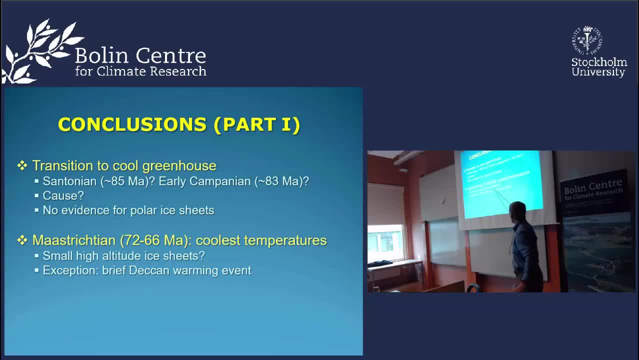 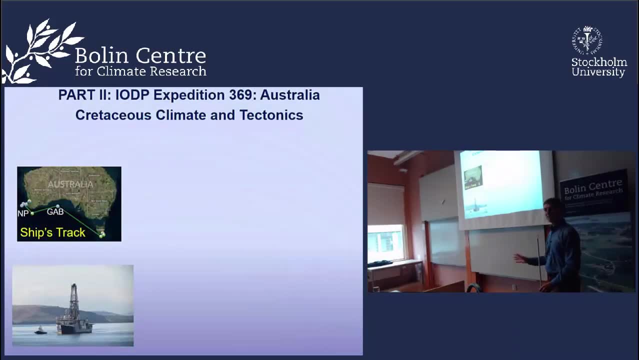 a little uncertain, but we know we have the coolest temperatures within this time for the cretaceous age, so now's the time. if you want to get up and leave, you're welcome. the second part is talk about the ocean drilling expedition, which is really in network to fill in the gaps of this climate curve. the expedition was one year. 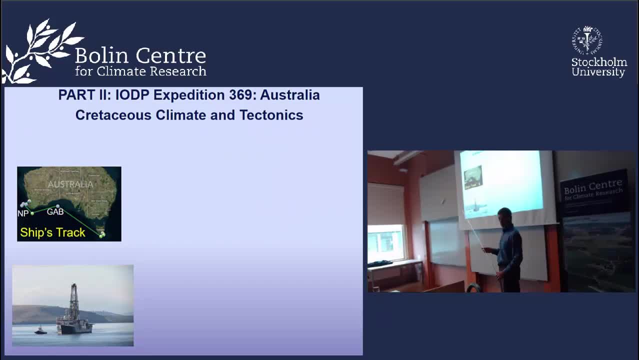 ago from right now. he started in october first. 所以, cranberrylc, we left hobart resolution, we drill their first site in the greatest running by 8 뜻. and then we drilled four sites: puneos in rio, tribute, introduction to climate change and desert husband막 carberrylc. 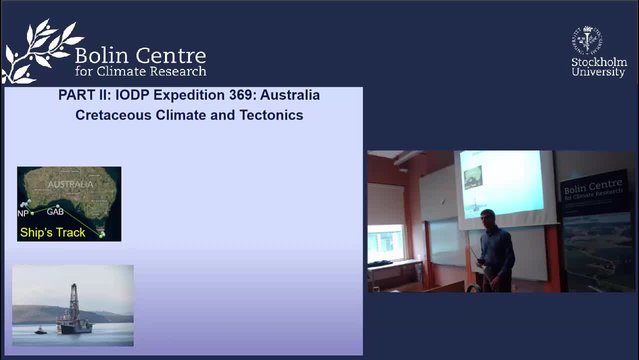 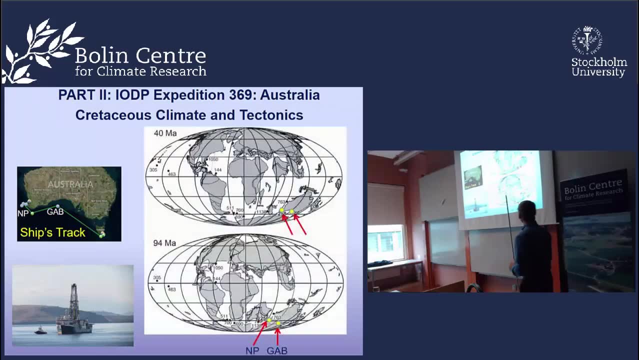 the world is now happening. outsiders area two, further elections and verz instruct us to CBC in the Mentel Basin off of southwest Australia And, again, to remind you, reconstruction of the continents. these are all high latitude sites, So all these sites are about 60 degrees south. 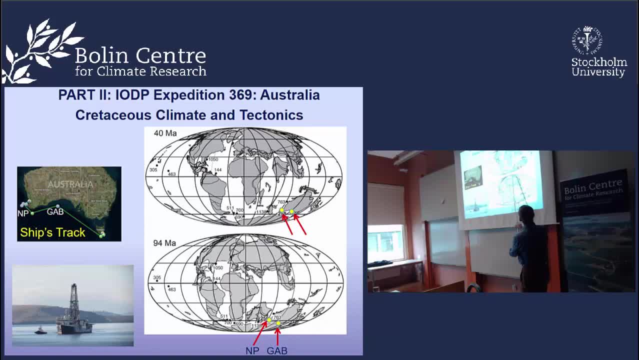 And so this is 94 million years ago. And then we wanted the record of when Australia separated from Antarctica and how the paleoceanography was affected By the deep and shallow ocean circulation in this region and how it also affected the deep circulation elsewhere. 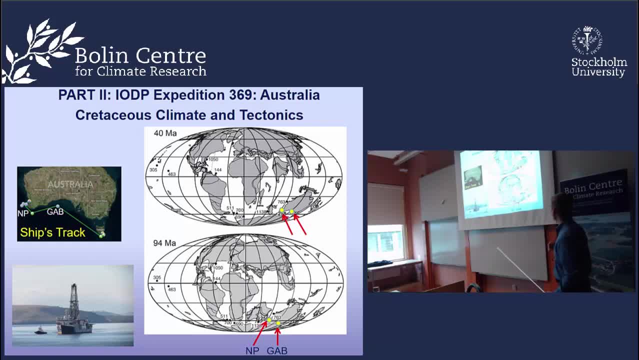 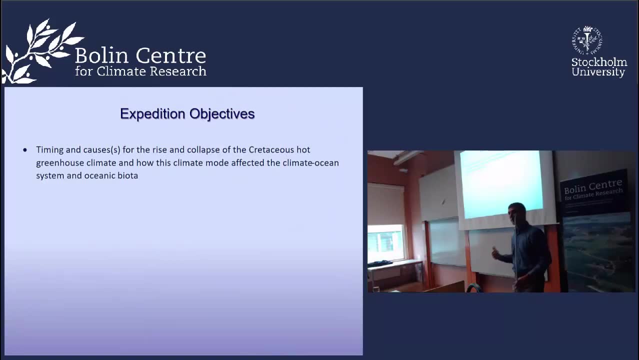 And so we're looking at a long-term Cretaceous through Cenozoic record of oceanography with separation of the Gondwana continents. So we wanted to fill in these gaps so that we can identify the timing of these temperature shifts. 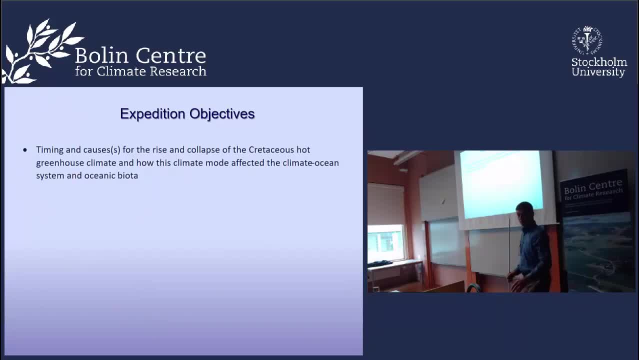 And see if we can identify the cause of those climate changes. We also wanted to look at how the role of productivity, temperature and circulation changed across what are called oceanic and oxic events, And I'll talk about this a bit more. 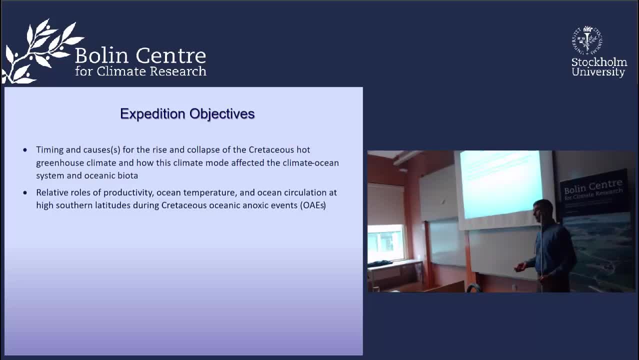 But basically these are times when the deep ocean temperature was very, very warm And the oxygen at the seafloor was used up And we had preservation of organic matter And you get deposition of what are called black shales, And these black shales are very widespread worldwide. 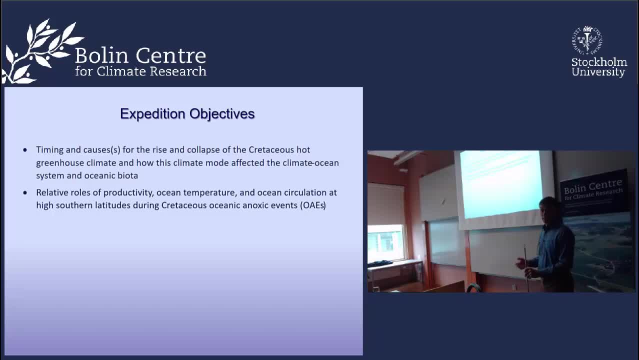 And that organic matter in the black shales are actually the source of a lot of petroleum, particularly in the Middle East. So these black shales have been controversial for 40 years, And our goal was to understand what triggers the deposition of these black shales. 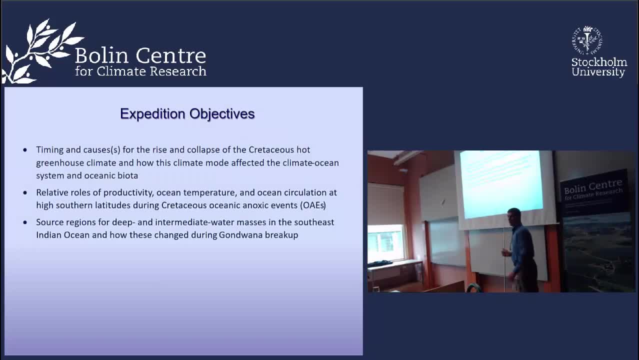 And then, as I mentioned, we want to understand how the deep and intermediate circulation changed as the Gondwana continents separated. We want to look at the oceanographic change of the Mentel Basin as the Tasman Sea opened, Looking at this seaway that opened between Australia and Antarctica. 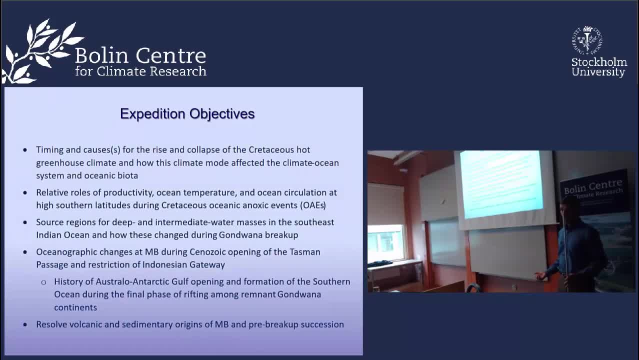 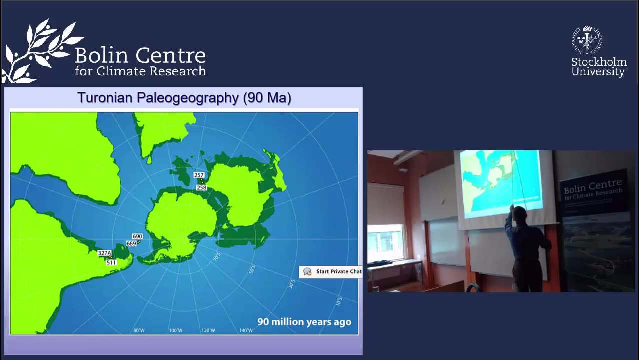 And then we also wanted to drill into the volcanic rock, underneath all the sediments, Get the age of the volcanic rock and understand their history of formation. So here's a reconstruction with a polar projection. Actually, at this time, 90 million years ago, land connected Australia and Antarctica. 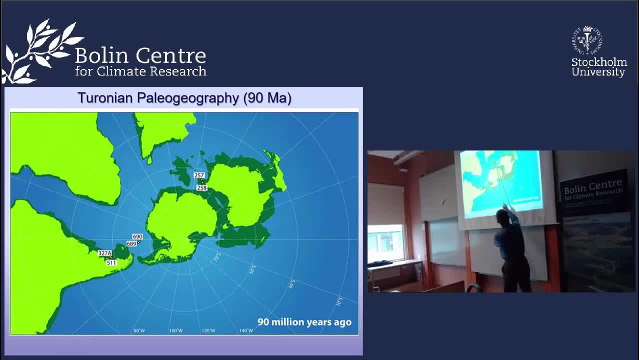 So there was no seaway here, but the seaway opened from the west to the east, And so it opened like a scissors pulling apart, with a deep ocean in the center And our site is right here, And so nobody has drilled this in deep sea drilling. 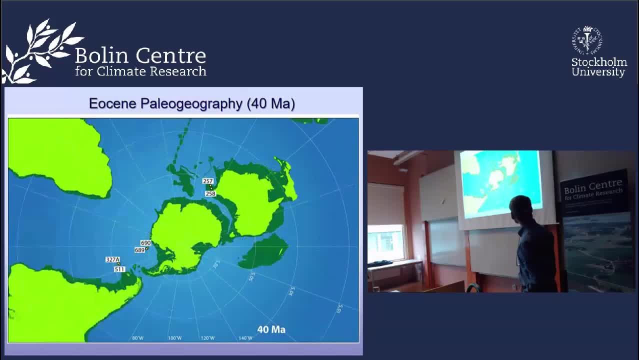 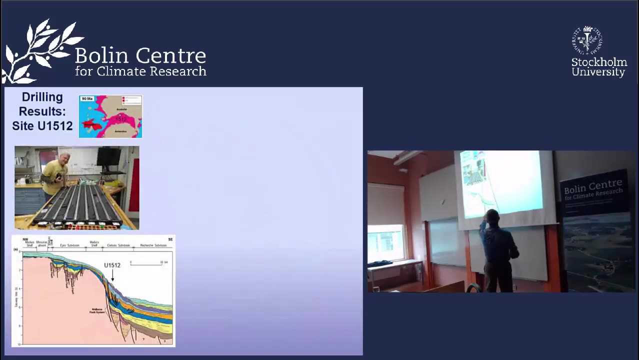 So we were looking at the history of this Cretaceous seaway And for the Eocene you can see how this is opening deeper And by the Ladyocene we have complete separation and deep circulation between the two continents. So the first site we drilled is site 1512. 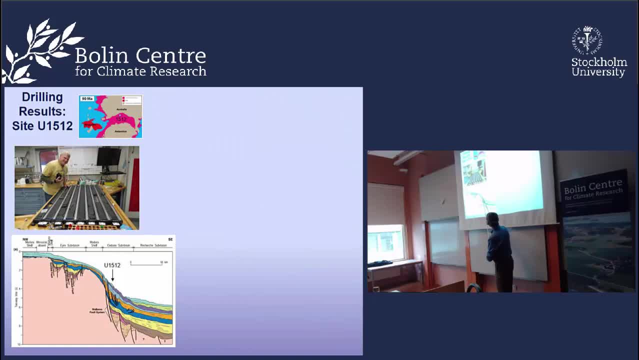 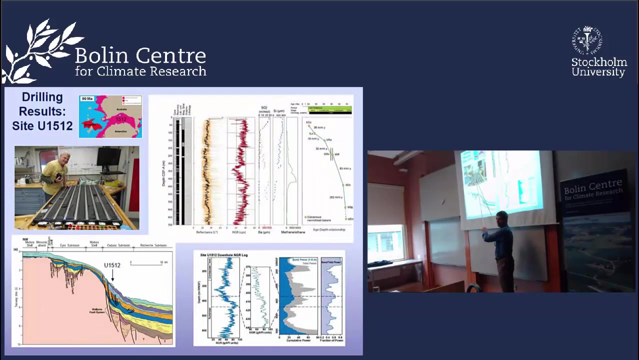 And this is on the margin of Australia- And so we drilled this site based on previous drilled wells, With the anticipation that we would get down at least into the Cenomanian age, back to about 95 million years ago. It turns out, almost all of what we drilled looks like this. 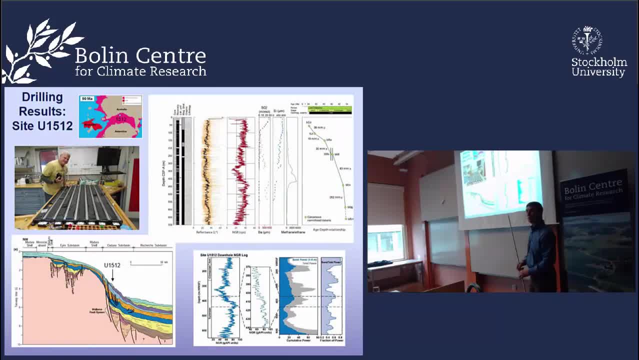 Very homogeneous dark mudstone, Pretty restricted in terms of the plankton, but the calcareous nanofossils yawn. David Watkins did a great job getting ages all the way through. This is an iconic foraminifera which I was studying and the shipboard scientists were studying. 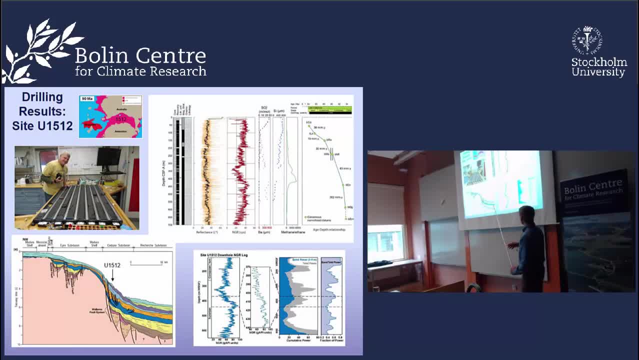 are very sparse and sporadic, But we have enough record, including some palynology, that we should get a very nice history of Cretaceous climate change in southern Australia. And what's interesting is some of these intervals are very cyclic, So we have Milankovitch scale cyclicity for some intervals. 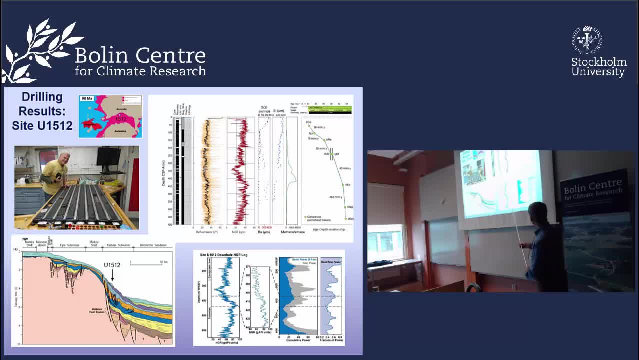 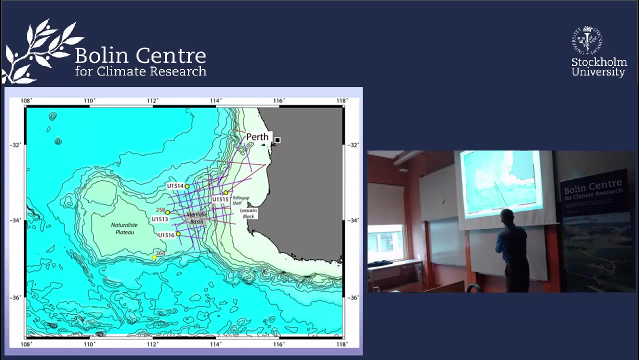 Very beautifully cyclic, Particularly showing up in our natural gamma logs and our magnetic susceptibility. So this site is going to be important, particularly for a regional study of Australia and for the study of the opening of that seaway. My particular interest, though, is these sites in the Mentel Basin. 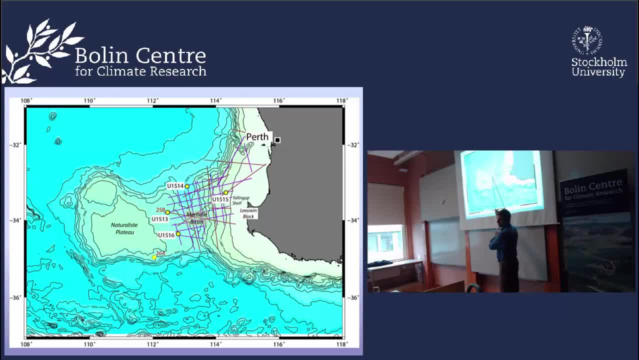 The first site that we drilled in Mentel Basin was a redrilling of site 258. So we went back to the same location where the drill ship was in 1972. And we redrilled that site with much better technology to get much better core recovery. 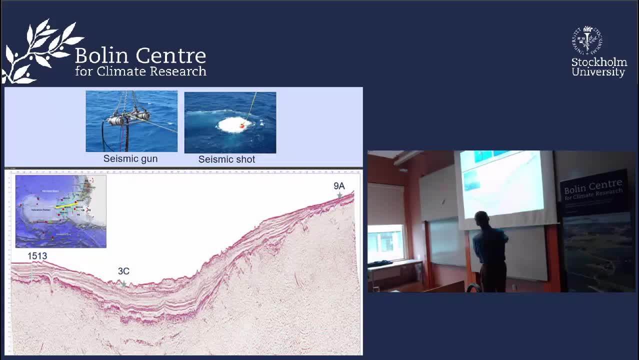 This is the seismic line going from the margin of Australia out to site 1513.. Here is what we drilled And we actually bottomed out in the volcanic basalt. We had 80 meters of basalt at this site, But you can see the thick pile of sediment which goes from- we had a bit of the Miocene to recent. 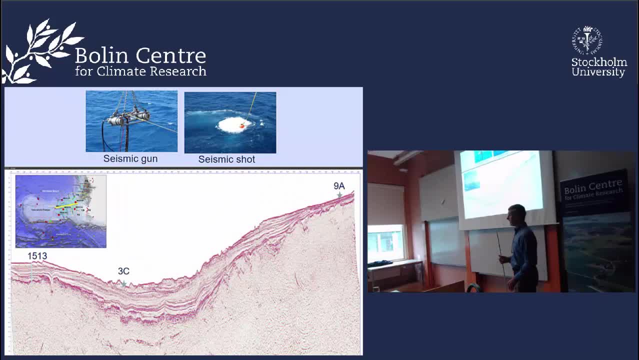 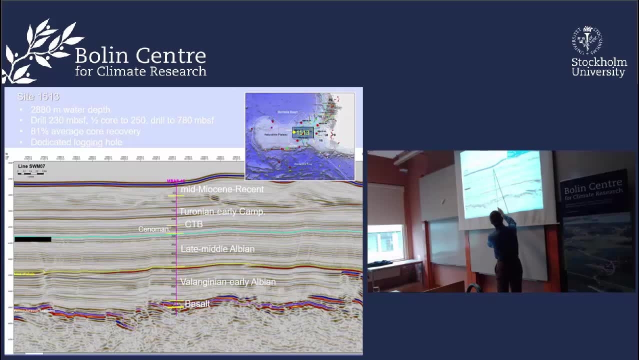 And then we jumped into the Cretaceous, early Campanian, down into the Albion, And that's what's shown here. So here we've got the Miocene, mid-Miocene to recent, And then there's a big unconformity. 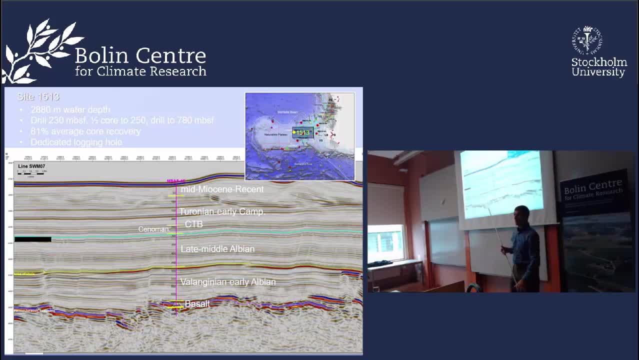 And we jump into the Cretaceous. We've got a beautiful cinnamony-tronium boundary, which is this, And this is that time when we get the shift in climate to the extreme warmth And then we get very long sequence of dark mudstones. 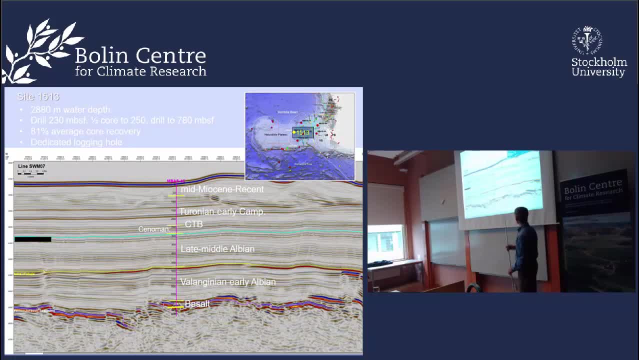 Very homogenous, with very few plankton foraminifera. But the great thing is, the preservation is good all the way down to here, And so with good preservation of the shells, we're going to get a very good temperature record all the way down into the middle Albion. 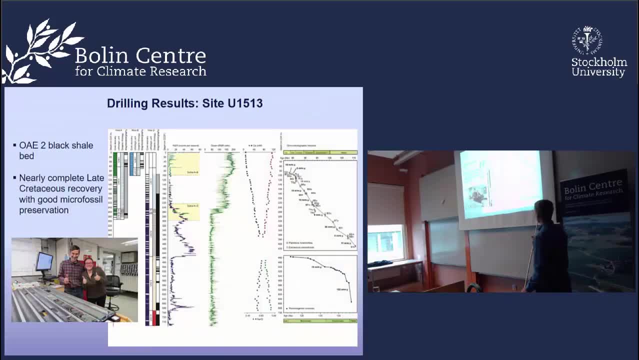 So we consider this expedition a great success. Here's our first black shale. You can see the dark black shale right here. This is at the cinnamony-tronium boundary. We actually went and redrilled this site, And so we've got two copies across the cinnamony-tronium boundary that we're sampling. 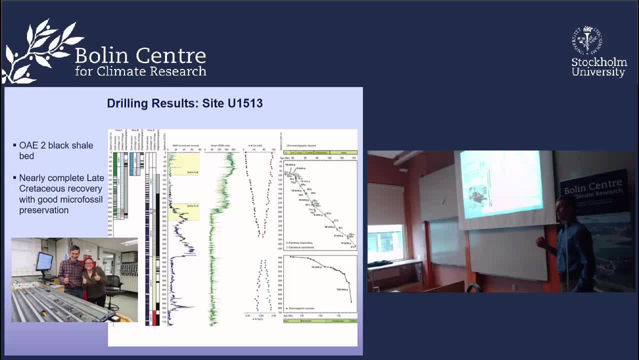 And one of the goals is to look at something called osmiomyces, Osmiomycetopes, through this sequence, Osmiomycetopes. the ratios of osmiomycetopes change when there's volcanism, And so a colleague in Japan, Junishiro Kuroda, will be looking to see if there's a shift in osmiomycetopes just at the time of the black shales. 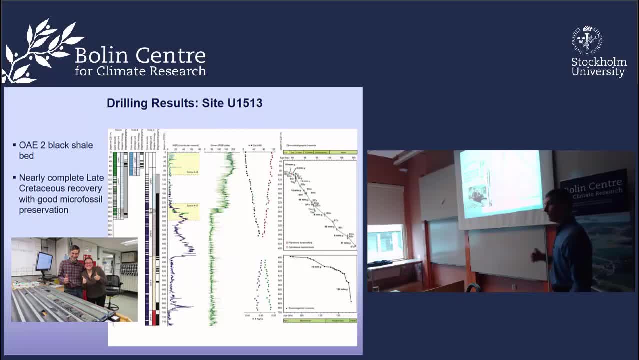 And, if there is, that will tell us that volcanic eruptions triggered the global warming across this interval. You can see we've got very nice Natural gamma records of beautiful logging, records from shipboard analysis as well as doing logging of the whole. Plus, we have a very nice age model to constrain the ages of all the samples. 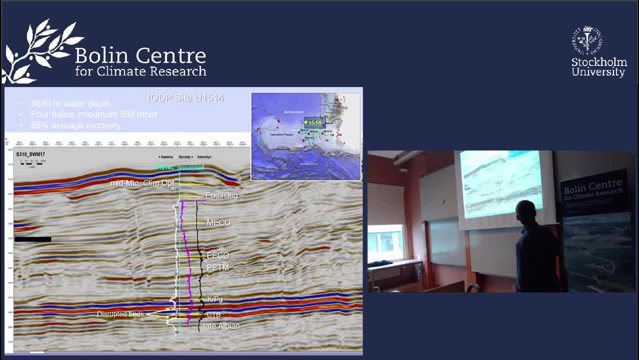 So the first site was a great success. The second site was on the northern margin of the Mentel Basin. It was also deeper, So it's about 800 meters deeper than the first site And by getting deeper of course we're going to get a deeper water signal of what the deep ocean was doing during the history of the opening of the Tasman Sea. 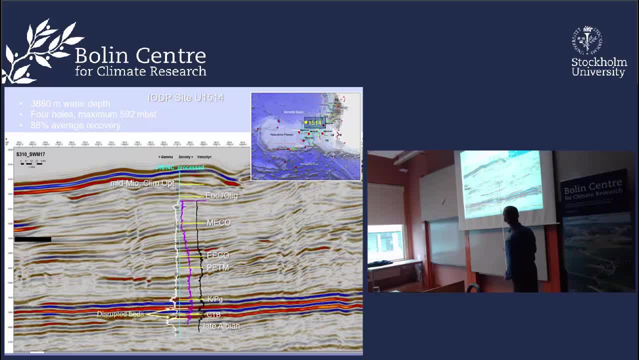 as well as the spreading of Kerguelen Plateau away from Australia. We expected to have a big unconformity again between the Miocene and the Cretaceous, But to our surprise we got a beautiful paleogene sequence all the way down, including a complete Cretaceous-Paleogene boundary. 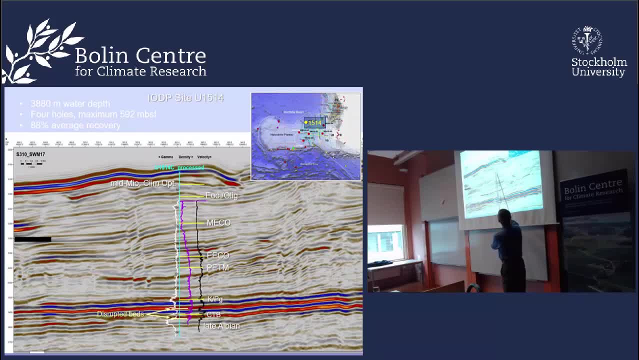 And so we hit all the highlights: Helen Eocene-Legocene boundary, We got the Mid-Eocene Climatic Optimum, Early Eocene Climatic Optimum, the PETM, and a Cretaceous-Paleogene boundary. Then we have an unconformity here. 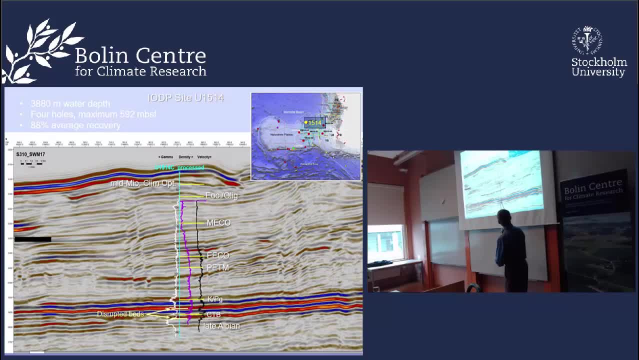 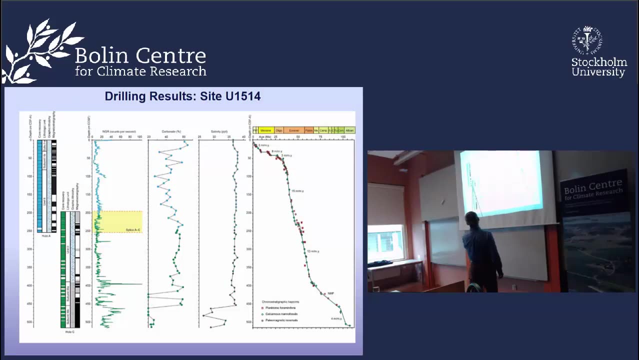 And we have a beautiful Santonian sequence and then a very weird Centomanian-Turinian boundary- I'll show. And then we get Lady Albion sediments. So we have two boreholes that overlap this part of the record, which is the Cretaceous part. 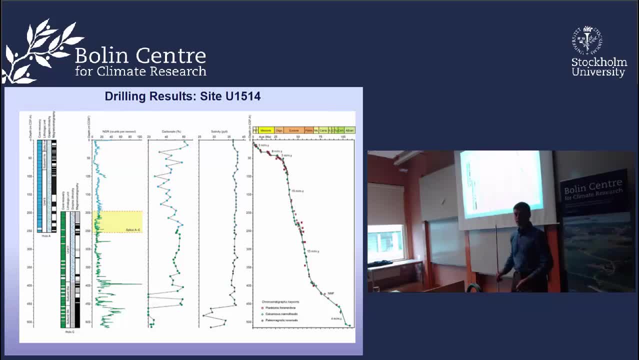 And very nice logging, as well as shipboard physical properties and natural gamma data and a very good age model showing the ages going down from Miocene to the Albion Core recovery. I should mention: The white represents unrecovered core And so the composite record, particularly across the Centomanian-Turinian boundary interval, is 100%. 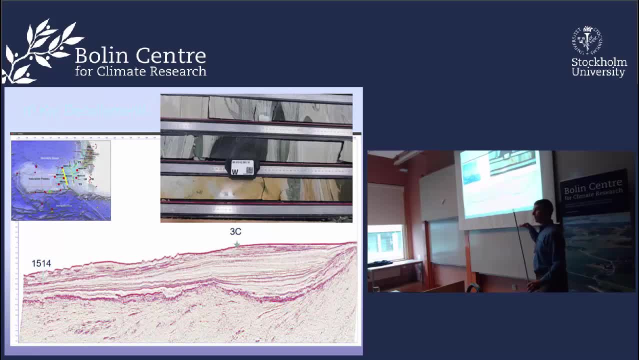 Well, we got this very weird sediment as we got to the Centomanian-Turinian boundary. So at about 94 million years we got this very swirly, beautiful, swishy sediment with black shales all mixed up. 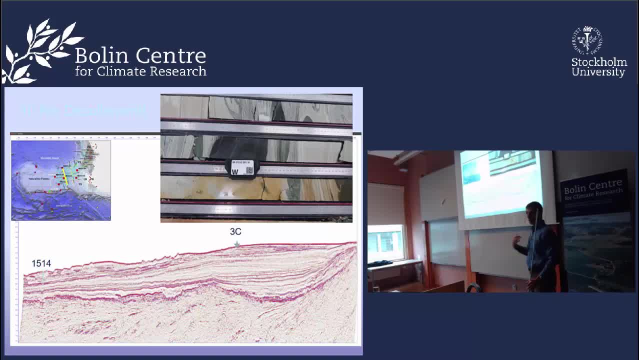 My colleague, Richard Hobbs, the other co-chief. I was a co-chief and then Richard Hobbs was the other co-chief. he's a geophysicist. He pulled up the seismic line across this part of the basin and he looked at all the instability here. 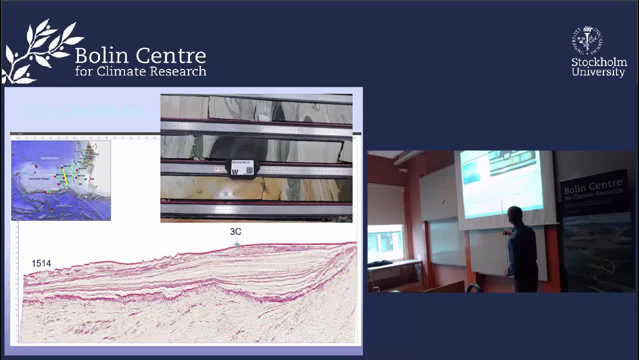 Even though this is a one and a half degree slope, this seems to be a big slip or a decollement, meaning the sediment slid down the slope, And so this is from sliding of the sediments. Everything just above this core is in place. 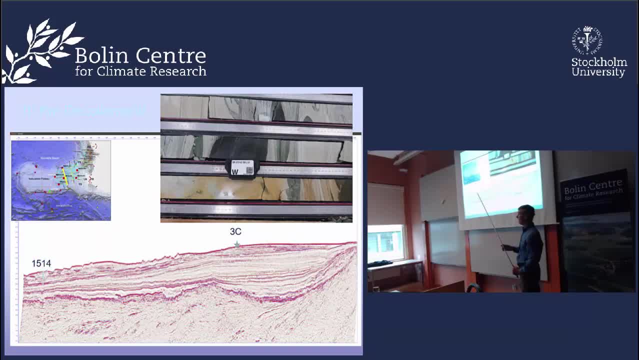 It all slid in place. We don't know just when it slid, And then everything below is fine, So it's very weird. It's very unfortunate too that the interval we were after Centomanian-Turinian boundary. 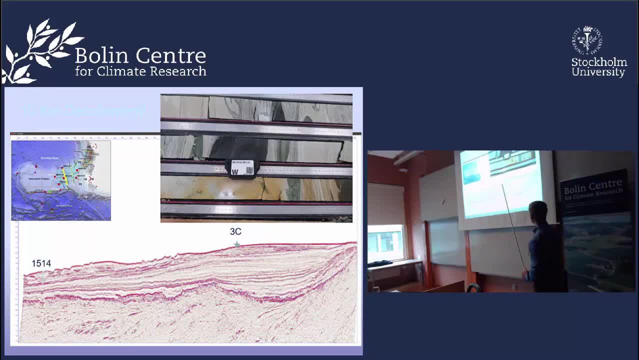 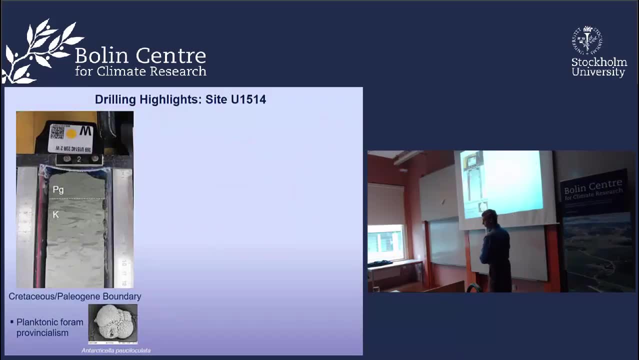 is all mixed up and we can't really study it to get the detailed record we want. Nonetheless, Helen, here's our Posse laculata. This is an early Danian marker, a species described from New Zealand just above the Cretaceous-Tertiary boundary extinction. 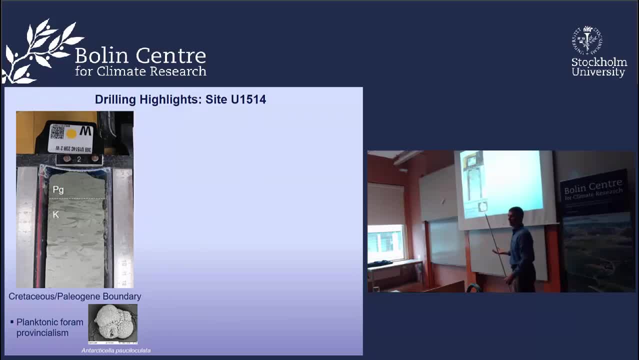 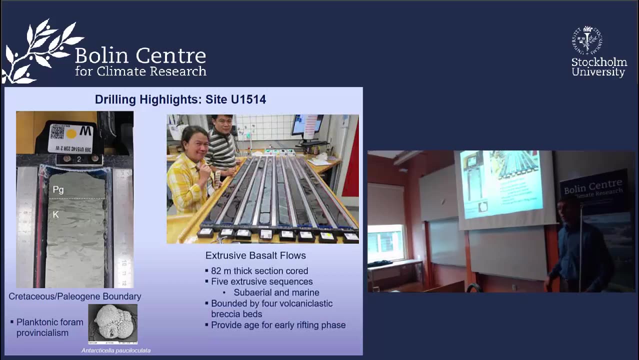 This is the boundary level, constrained by planktic foraminifera and calcareous nanofossils with a bit of bioturbation, But it's a very complete boundary. And here are the basalts that we covered. The basalts are fresh enough that we should get some very good radiometric dating. 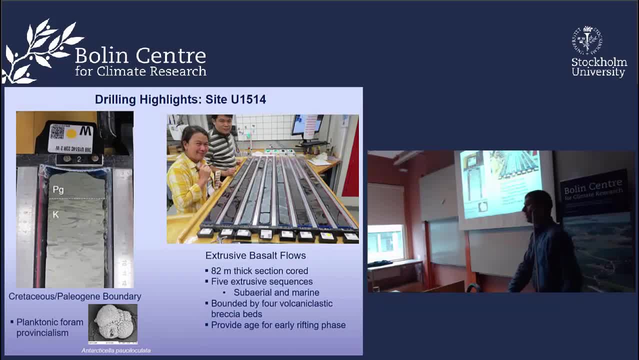 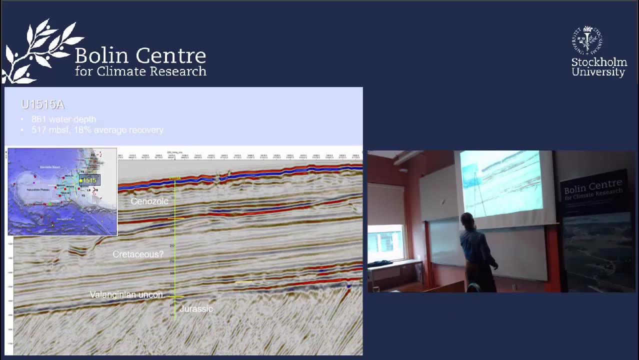 to determine the age of when those basalts erupted. And also, some of those basalts were red-colored, which means they were subaerial, which means they erupted above the sea level. So then, the shallowest site was 1515, right on the margin of Australia. 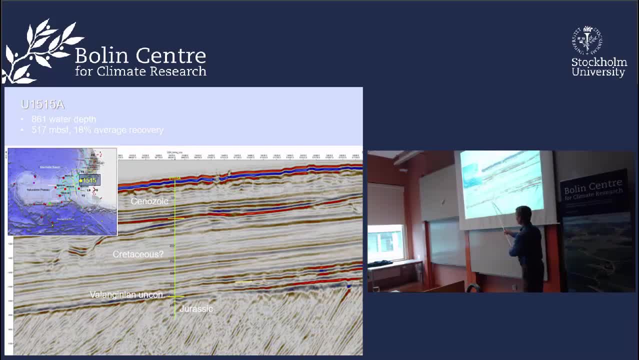 The goal there was to date these highly dipping sediments, And we also wanted to find out what these sediment ages were here and get the whole history. So we did a lot of study of the shallower water deposition of Cenozoic through Cretaceous. 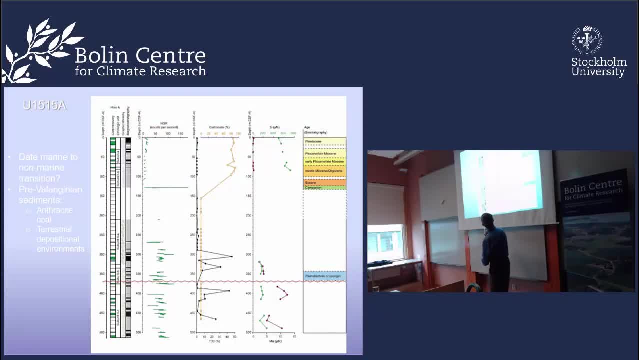 It turns out, there's a lot of loose sand in these sediments, and so the white dominates the core recovery. In other words, we had very, very low core recovery. I think it's averaged 15% because of these sands. So poor recovery, but the intervals that we recovered were enough to provide age control. 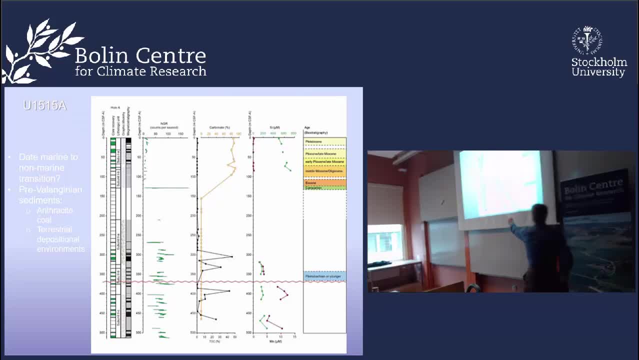 And so we have these age windows For all of this interval. the age control is going to be determined by palynology And I'll talk to Vivi about maybe whether she would get some samples to help with some of this. So for those who are trying to understand the tectonic history of the margin, 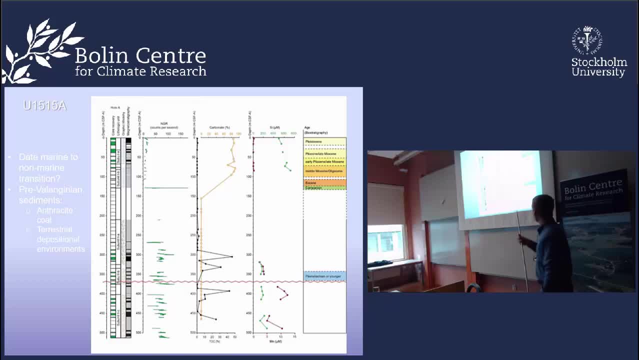 they were very happy even with this poor core recovery. There were coals, We've got coals down here. There's also coal down here And the age we got from palynomorphs in samples from right here suggests Jurassic age. 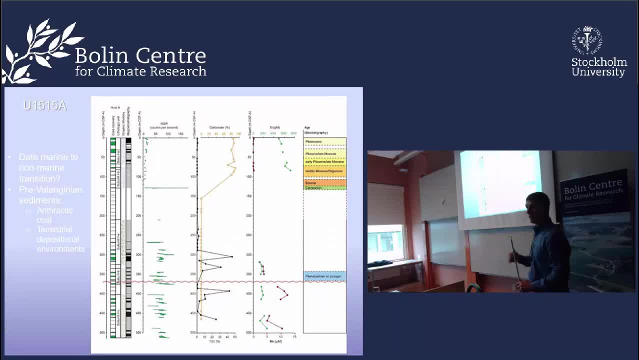 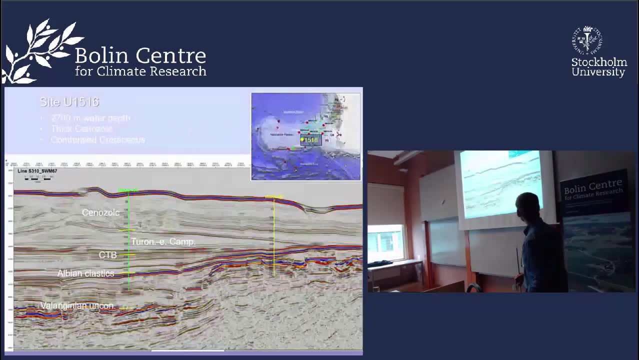 And so this helps determine the timing of the tectonics, and we know at least, the dipping beds are older than Jurassic. The last site we drilled- 1516, is shown here, And it's to the south of the site 1513. 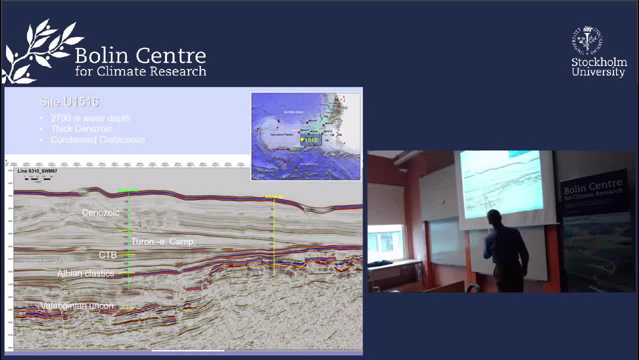 which I talked about earlier. This is the record we got. These are the seismic, very stable stratigraphy all the way down. We have a cenozoic record. I'll talk about beautiful cinnamony-trony boundary And then we get back into the Albion shales again. 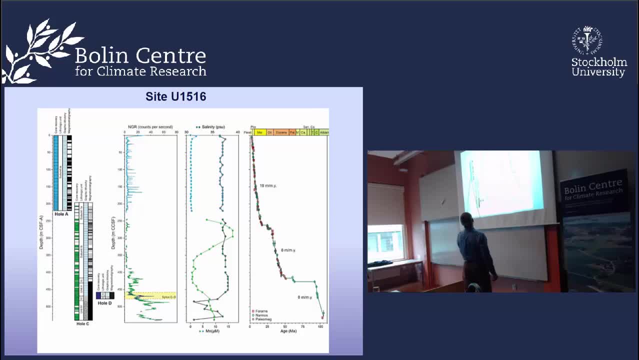 You can see 100% recovery for the first part, which is cenozoic, With the nonconformity in the Oligocene reef interval of the Eocene, And then we jump into the Cretaceous, down here. Our cinnamony-trony boundary is down here. 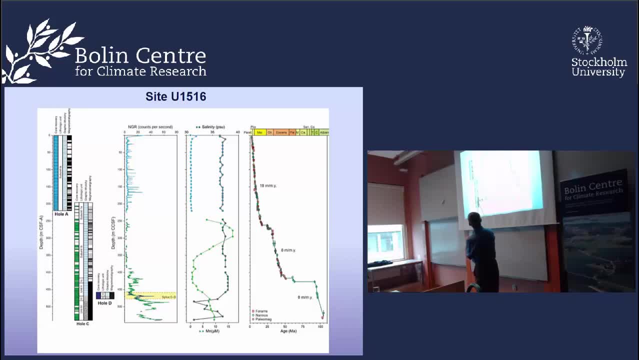 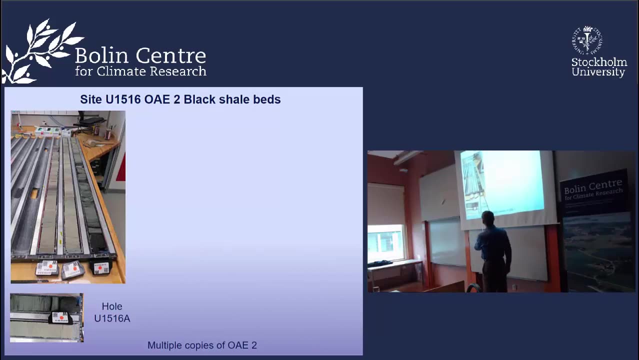 So we have two copies of the cinnamony-trony boundary at two holes And 100% recovery at the second hole. So we're very excited about this. The first hole: we got the black shale. The black shale was at the bottom of the core. 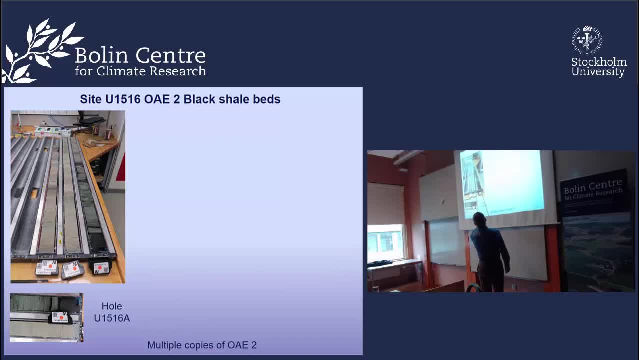 And you can see there's actually not just one black shale. There's a thick one, There's another black shale And another black shale. This interval right here is very carbonate poor, So there's almost no calcareous nanofossils or foraminifera. 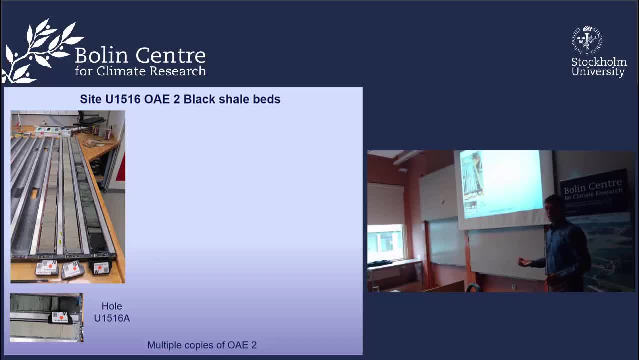 Which is weird. It seems to be very siliceous, full of silica, Which suggests high productivity of siliceous plankton, Which suggests this was driven by volcanism and high productivity to cause the black shales. But we wanted another copy of the core. 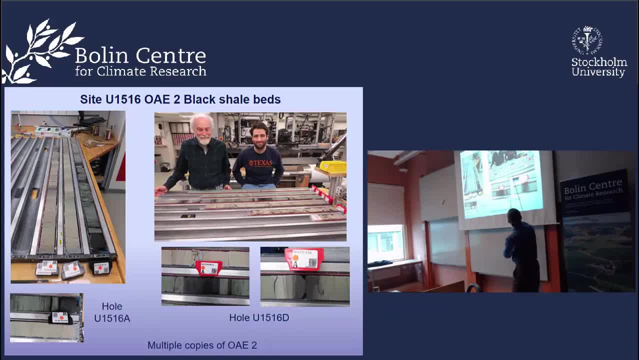 And David Watkins and Gabrielle are very happy Because here's the black shale in the middle of the core, Again with the black shale here, Another black shale here And here's close-ups. So these are laminated, Meaning there were no organisms burrowing the sediments to mix the sediments up. 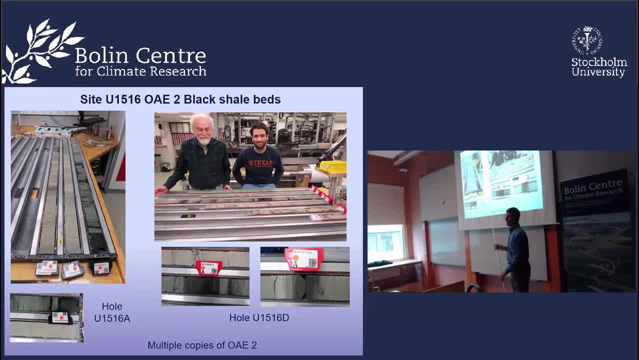 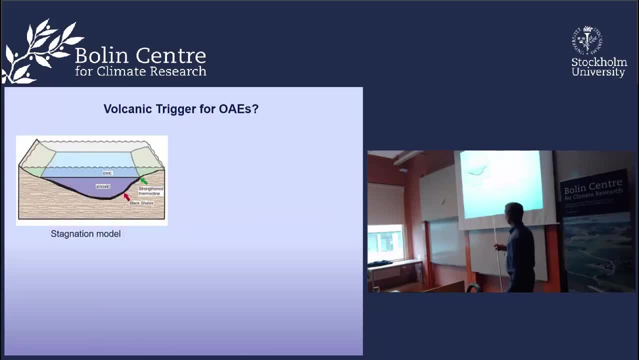 And no oxygen on the seafloor at this time, A very weird time when the ocean goes anoxic. So, as I mentioned, there have been controversy about what causes these black shales, And one is the stagnation model Where, basically, you have no ocean circulation and no replenishing of oxygen in the deep water. 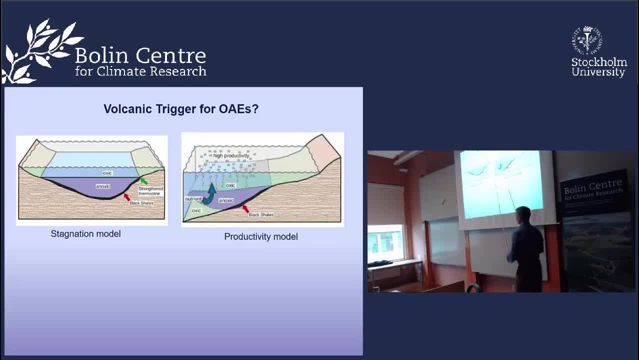 The other model is called the productivity model, Which suggests you have nutrients getting into the ocean, Lots of plankton productivity, Lots of organic matter that sinks to the seafloor. That organic matter overwhelms the oxygen on the seafloor And you get the black shale deposition from that. 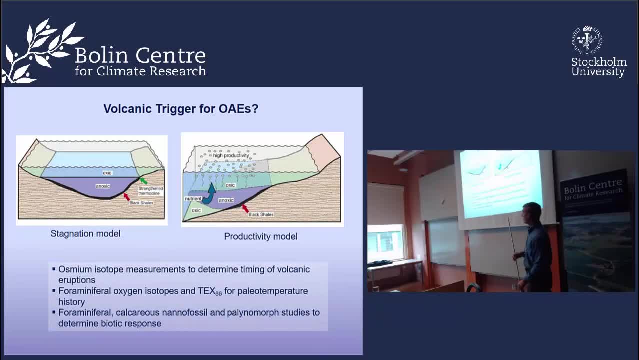 And so, like I said, we're going to use osmium isotopes to determine whether the volcanism is the trigger And then, above and below the black shale intervals, we'll have constraints on the temperatures And how they change across this boundary interval. 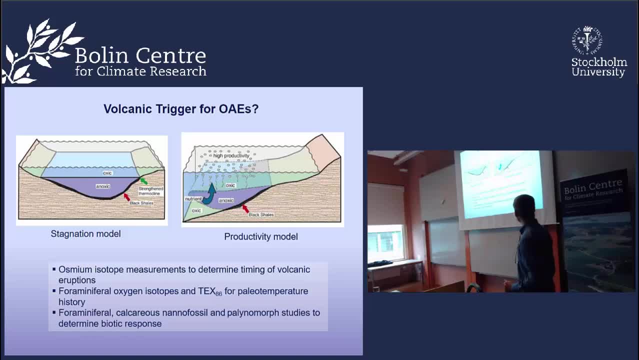 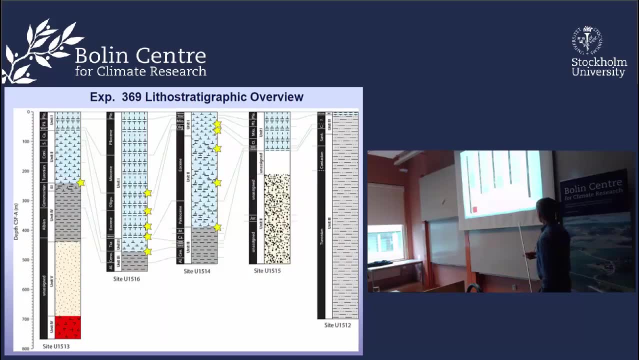 And of course we're also going to look at the biotic changes To see how the ocean biota were affected by this warming. So to summarize all the different sites we drilled, We've got these critical intervals. We covered nice Centromanian-Tronian boundary here. 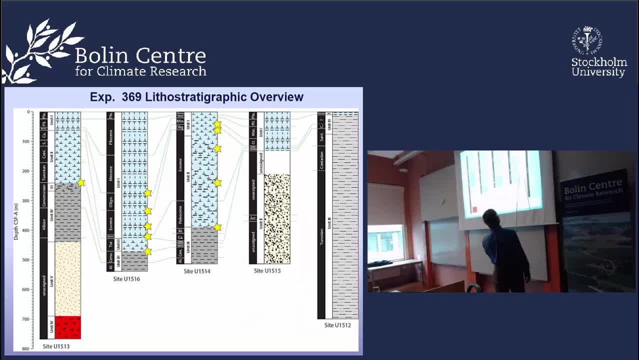 And another beautiful Centromanian-Tronian boundary at- sorry here- 1516.. And then at 1514 we've got this beautiful Unexpected paleogene record with lots of critical intervals. It'll be studied in great detail. So Kirstie Edgar is doing this work. 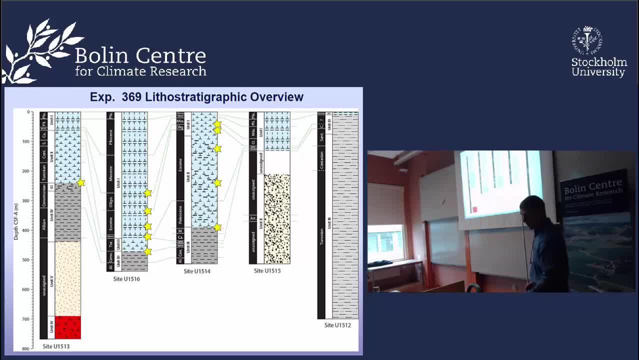 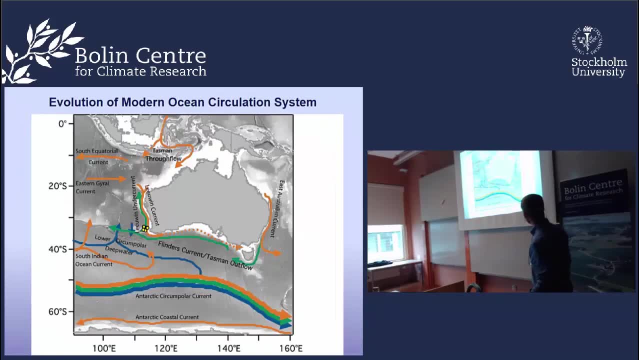 You probably know that, Ellen. So actually we came off the ship achieving more than we expected for the original objectives of the expedition, Some of which will be some detailed reconstructions of the ocean circulation here, Because we have beautiful cyclostratigraphy in the Miocene. 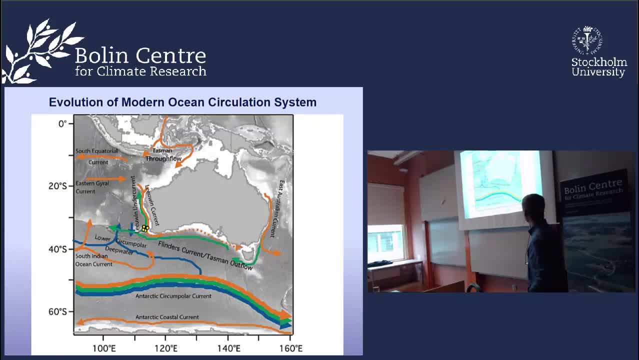 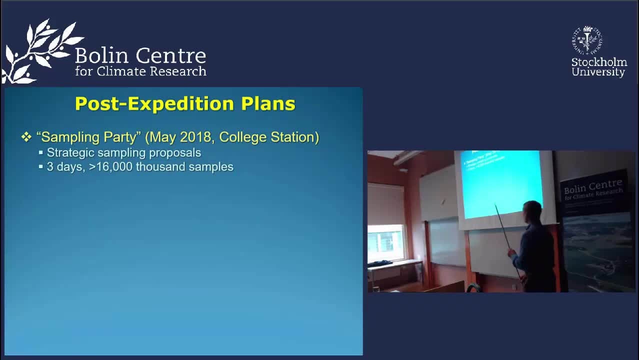 That we didn't expect to get. That's going to tell us a lot about changes in the climate and oceanography. So in May we went and sampled the core. We took over 16,000 samples From all the cores that were obtained. 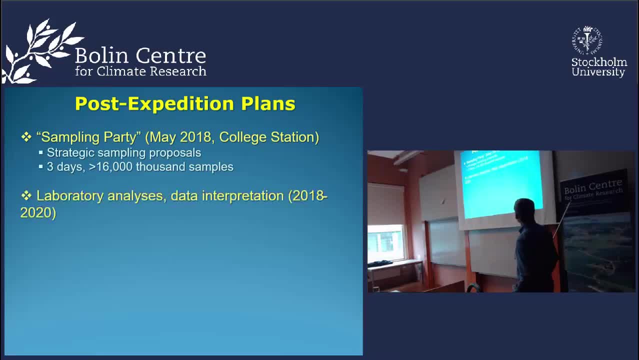 We're now in the middle of doing a lot of laboratory analyses And then we are Whoops. Okay, So we're doing the age constraints, The biostratigraphy, And then all the chemical analyses and the sedimentology is happening now. 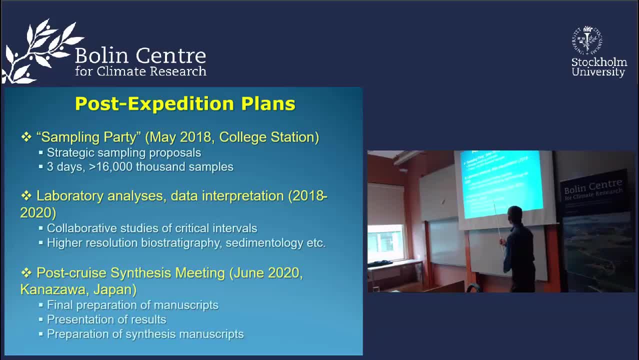 And then in May of 2019 we'll meet in Kansawa And whole shipboard and shore based team will discuss results. up until then We'll continue our collaborative discussions And then we'll have papers being published from that point Forward. 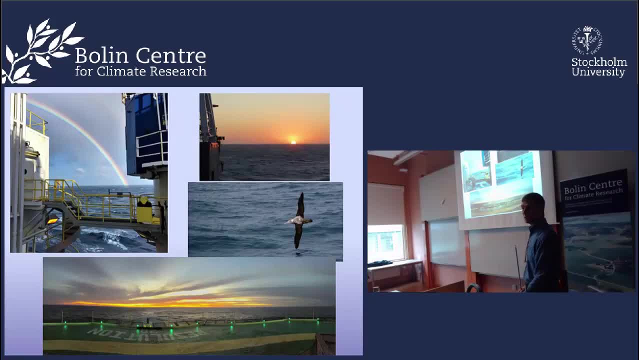 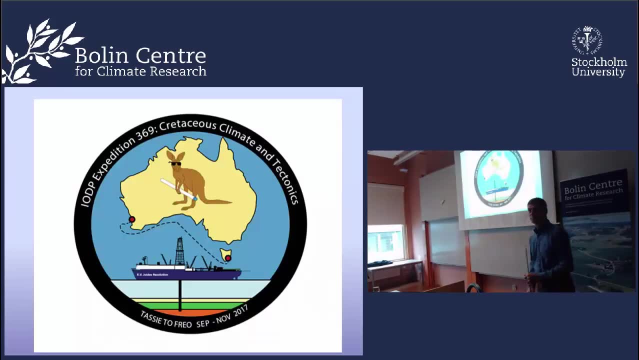 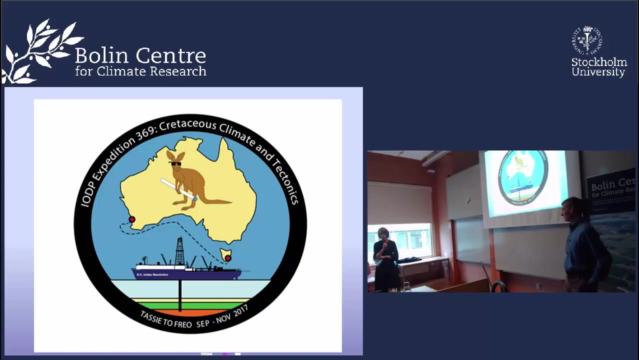 So with that, I'll end with some pretty photos from the drill ship And be glad to take any questions If you have. Thank you. So the first one is: what's the temperature of the ocean? Which is the temperature of the ocean? 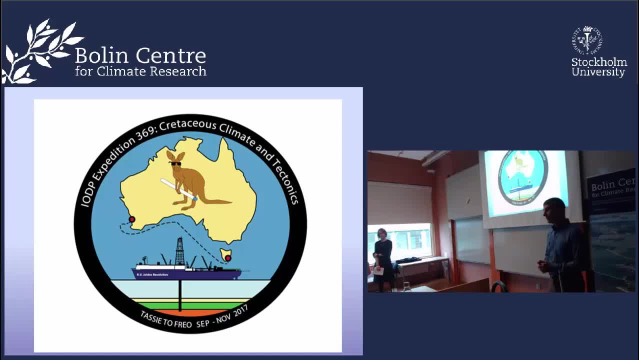 Is it a low or a low temperature? We're seeing a lot of both. I have a couple of questions, So the first one is: how much do you think it's going to affect the ocean and how much will it affect the ocean? 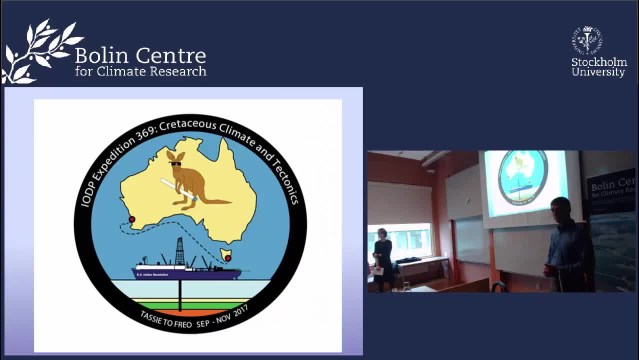 What's the temperature going to be? And then the second one is: how much of the ocean is going to affect the ocean? was it austral summer temperatures? yeah, so you know, plankton forums have a seasonal cycle of when they're most abundant, and so some reproduce in the 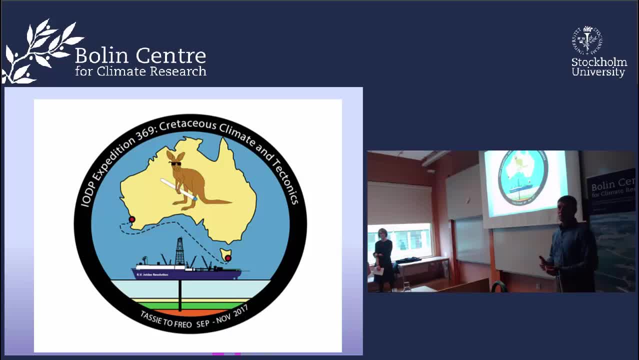 spring. some reproduce in the summer. for these things you never know when they're reproducing because they're all extinct. I think you can assume they might be summer maxima, but when you consider the benthic temperatures, those are going to be averaged and so the fact that we're getting values of minus 2.2 per mil. 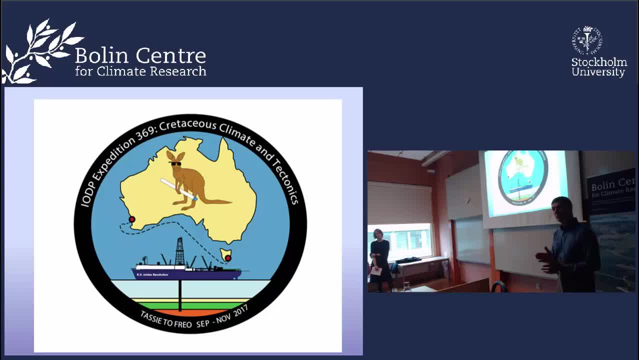 minus 2.6 per mil consistently for different multiple species of benthic, for a minifera suggests those deep waters are really really warm consistently through the tronion. so our peak values are right in the early to middle tronion. so, like I said, 2.6 minus 2.6, 2.2. but they say around minus 2 per 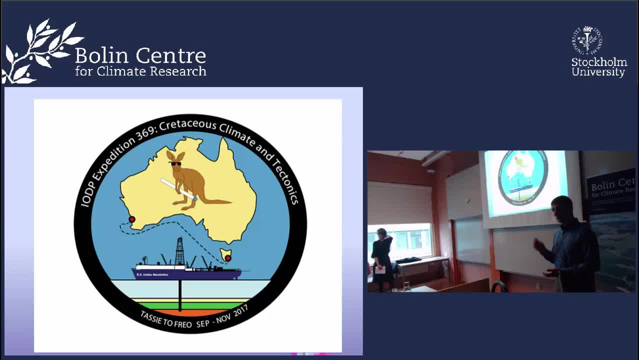 mil might have 1.8 per mil all the way through the santonian. so this is a really long time for extreme warmth. and to sustain this extreme warmth you got to keep pumping co2 into the atmosphere, because it's constantly getting buried and so if you're pulling out the co2, it should be cooling, so you 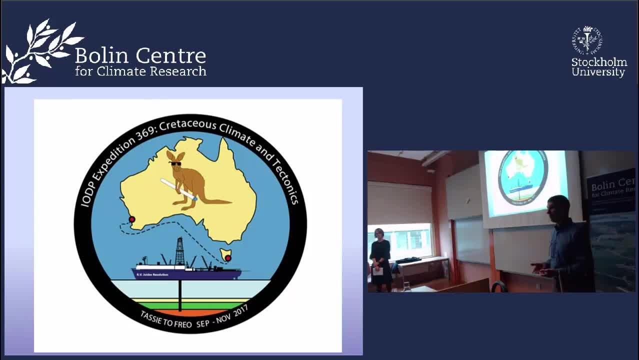 have to have another source of co2 that's keeping the climate warm, and this is what we're looking for. do we have sources that can explain how this, this high co2 earth, is maintained? and Stefan thanks Brian. his name, bill hay, recently put forward the idea that in the 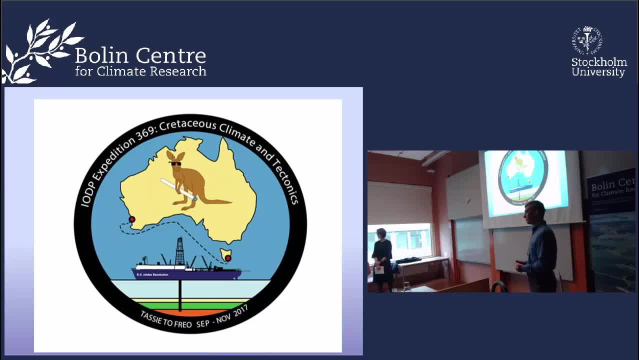 cretaceous, you had huge lowlands, because there were virtually no matter of, well, no mountains compared to nowadays world, and that in these lowlands you could store a huge amount of fresh water. actually, well, you could saw a huge amount of water, which a would produce a lot of fresh water and it would produce a lot of water. 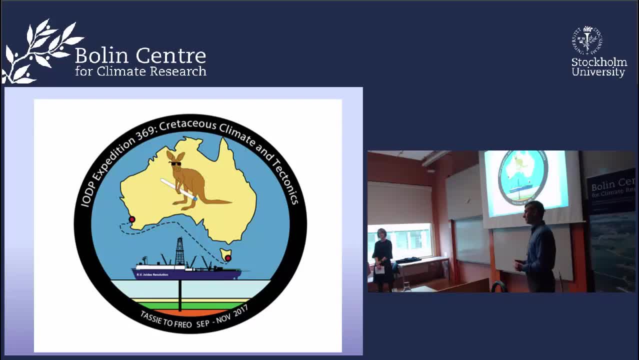 vapor, which is a good greenhouse gas, and B it could be responsible for for sea level changes, because for some reasons, I mean sometimes the water could go back to the ocean and sometimes it could just be stored in huge lakes or meandering rivers. you comment on that, sure? so, for one thing, I think the 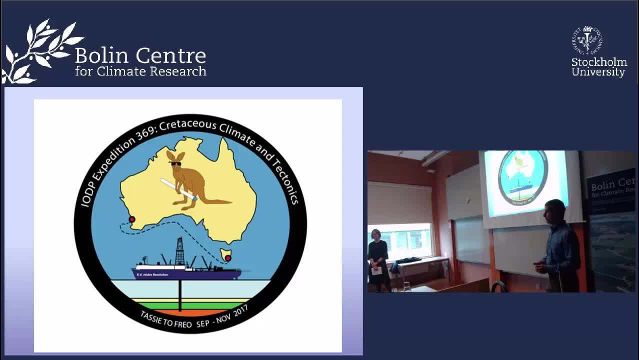 hydrological cycle was very cranked up during this time. so you imagine warming the ocean surface to 28 degrees C or warmer. you can get lots of huge storms which is going to move lots of precipitation, and so I think continental interiors had lots of rainfall. I know that, Bill. 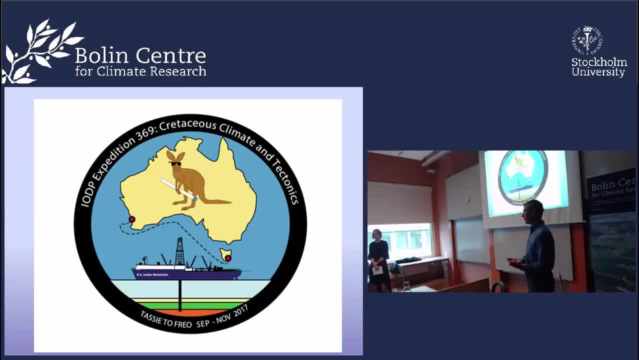 Hayes thesis is based on his interpretation of somebody's publication on a patasaurus- the big sauropods- and the only way to support those big sauropods is for them to sort of hang out in lots of water. and not everybody agrees with that interpretation. 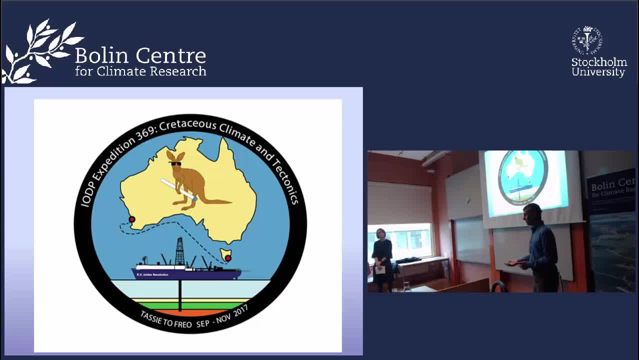 it's also based on: how else do you change sea level unless you're storing it on land? talking to bill Bill Hawk below Hawk, he still thinks it's a very small percent of the sea level curve because the volumes still won't add up for groundwater storage. so I'll let the professionals on sea level fight that. 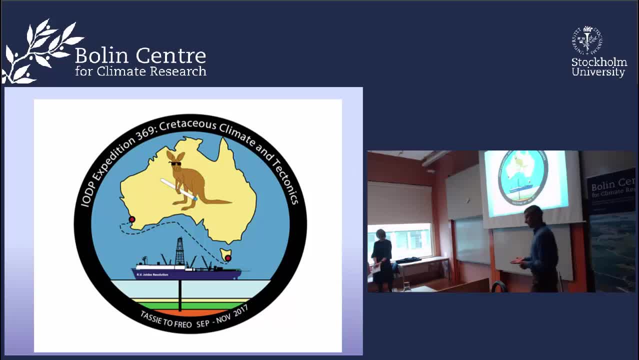 out. I was just skeptical on the sauropods story- talk to my dinosaur colleagues. but one of the neat thing Bill Hayes done is remind us that the Cretaceous world was completely different from today, and in one of his publications he talks about the eddy ocean and the fact that we don't have the normal Haley. 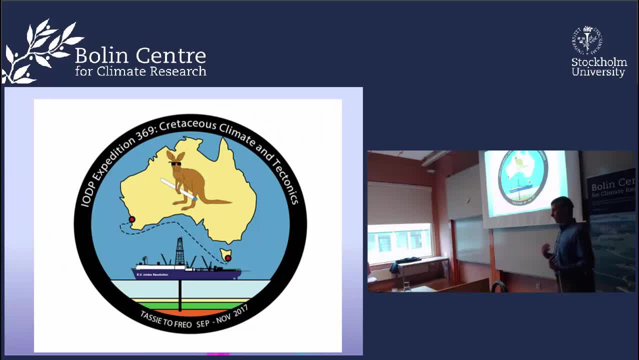 cells, Hadley cell circulation, that we assume and he thinks are just lots of eddy cells that are moving this moisture and moving the the temperatures and making it much more equitable between low and high latitudes. so he's got some really cool ideas. I'm not quite on board with with that one, but maybe there will be more evidence for. 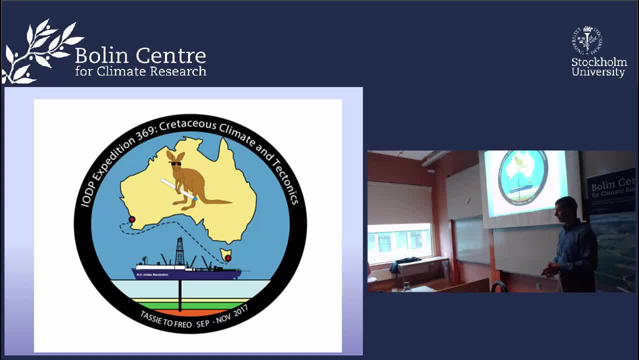 it more of a comment. thank you for a great talk. I'm always envious to see such high resolution data, of course. I just want to comment that I was a co-author on a paper by Chris Mays, who was a great writer, history writer on the geive way, and just wrote about the 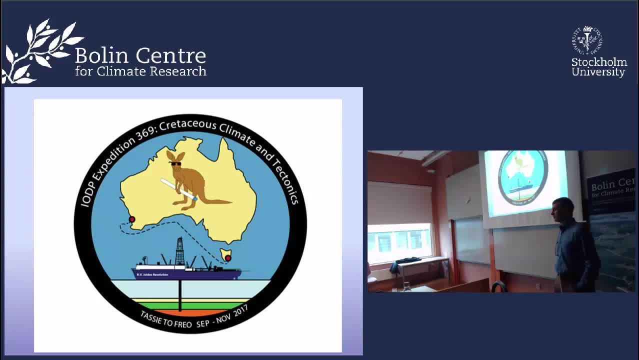 A record from the Chatham Islands, which was about 70 to 80 degrees south during this time, and we have unfortunately just one interval, but it's in the late Sinomanian, where we reconstructed CO2 using ginkgoitis variances, which is kind of the gold standard. 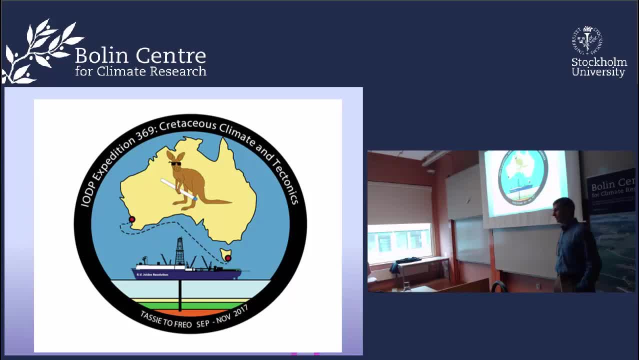 Ginkgos are the gold standard for CO2 reconstruction And we found concentrations of between 1150 and 1350 ppm, So I'm hoping you might add that to your. Yeah, so I use a curve compiled in Nature Communications Author's name. I'm forgetting. 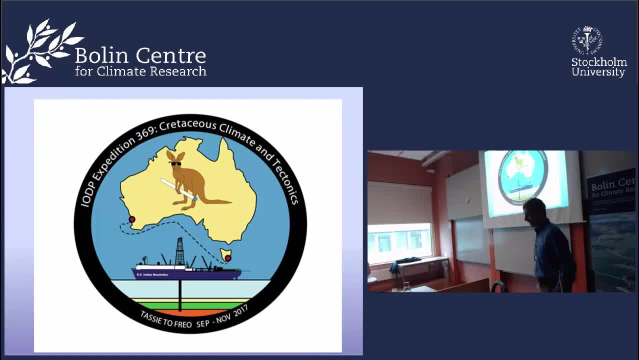 Thank you, And that must not have been on that curve because, Yeah, that's from 2016, and the paper is from 2015,. so you probably missed it. I like that reference. That sounds really good. Was that with Chris Hollis also? 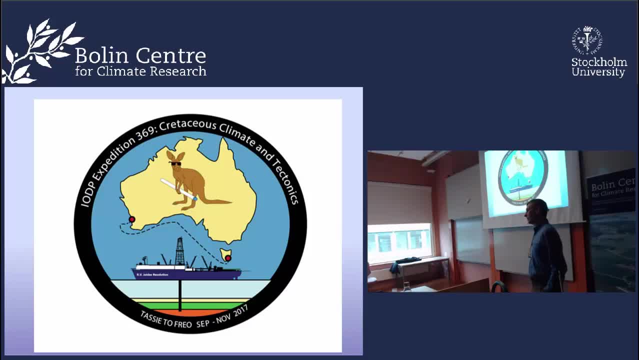 Yeah, Okay, Okay, yeah, Excellent, Great, Cool, Cool, Okay. You know, what we go by is a general assumption that I think is pretty reasonable, and that is if you're going to have normal open ocean plankton. 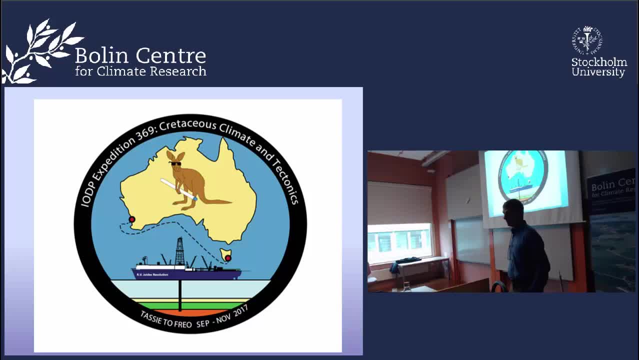 you're going to have pretty much normal open ocean marine salinity, And so the salinity itself. I think whether it's 33 ppt or plus or minus a few hard to say. I think the big unknown is the isotopic composition of the ocean. for this time, 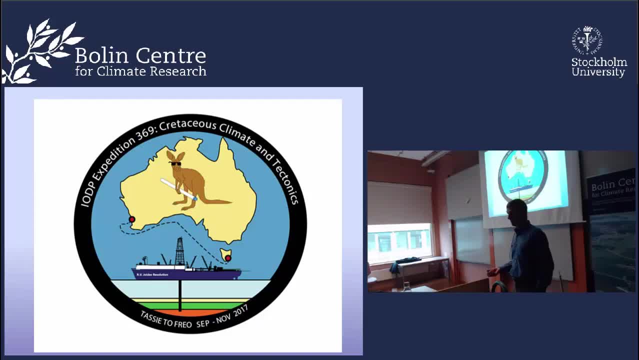 and our assumptions for estimating the temperatures of the Cretaceous. The modelers for the isotopic composition assume sort of relative weathering and sort of a relative cycle of mixture between terrestrial sources and oceanic, And so I'm going to go back to the ocean mixing and say that ocean salinity of the Cretaceous. 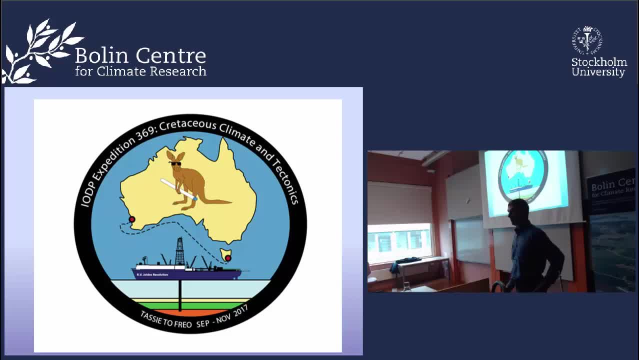 is really no different than today. So I sort of can only go by those models and those assumptions, And it's something we need to keep in the back of our mind- that is this a safe assumption? But the reality is that we're dealing with again, benthic foraminifera that are representative. 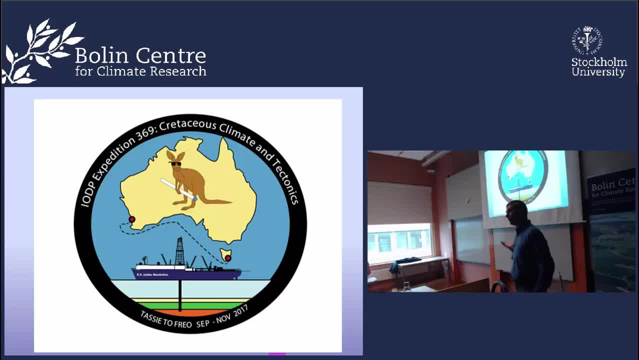 of a very long-term mixed ocean record, Even if you don't believe the really warm values of the planktics, which seem completely unreasonable. And I would say there's a salinity factor for the high latitudes. So there's Rayleigh fractionation, which is going to distill out the oxygen-18, so that 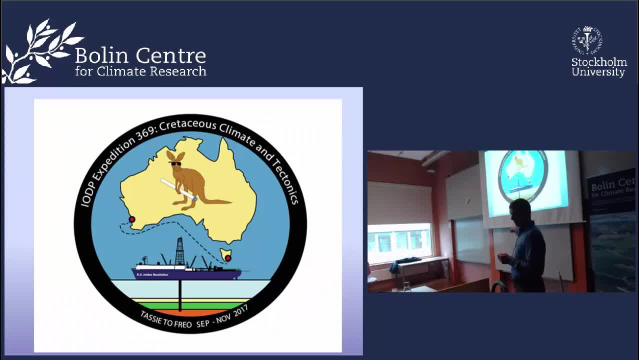 you get more oxygen-16 at high latitudes. So that's in effect in the plankton. And then there's probably a salinity factor as well because of higher precipitation at high latitudes. So I agree, The planktics were probably overestimating the temperatures. 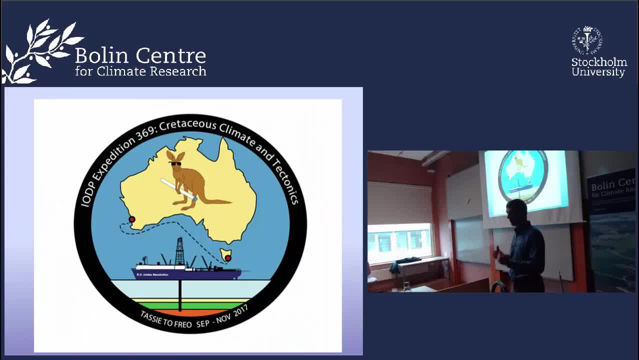 Still the benthics. that's, I think, what you really can trust in terms of a long-term temperature history of the Earth And the fact that it's consistent in both ocean basins reinforces our determination that this is a switch to an extremely hot greenhouse climate. 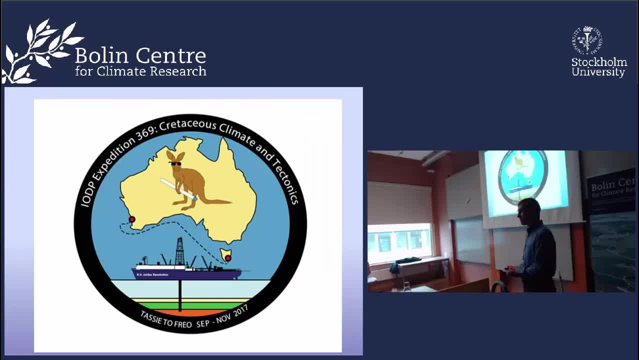 And the terrestrial record? yes, Right, Right, Dr. Really interesting question. Thank you, Yeah, So the type exchange is the main pathways for, would you say-, Dr, When the temperature changes, bars and bars are cut off? Yeah, 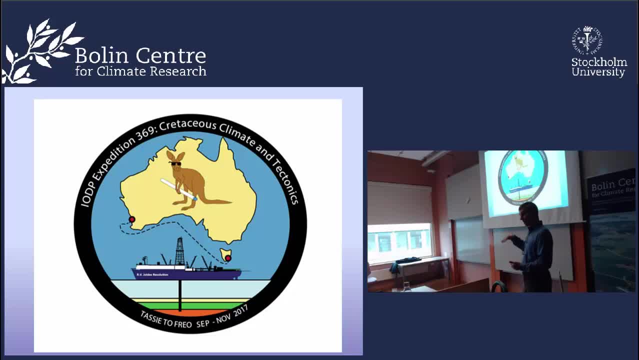 Good question. We don't have control on that, And one of the questions you have to ask is: why would there be- assuming there is- an abrupt shift to the sentiment in- mondrian boundary? why would there be a very abrupt increase in methane at that time? large volume volcanism causing CO2 to pump into the atmosphere. I don't know what the source of a sudden eruption of methane would be, unless all the dinosaurs suddenly started passing gas at the same time in greater volumes than ever before. So the hydrologic cycle would have 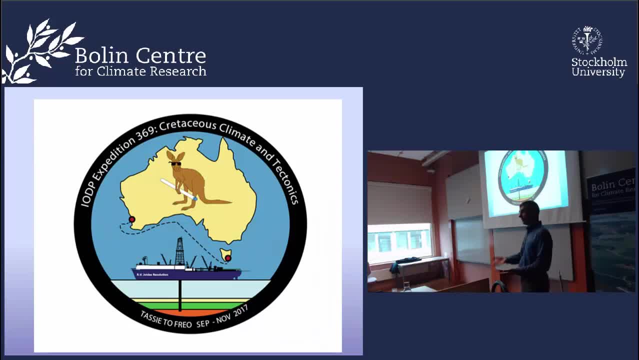 to switch to have storage and then sudden release. So I think all of our assumptions need to get put on the table and everything needs to be questioned, And questions like this are also worth pursuing. The challenge is figuring out what are the proxies, to come up with reasonable interpretations that 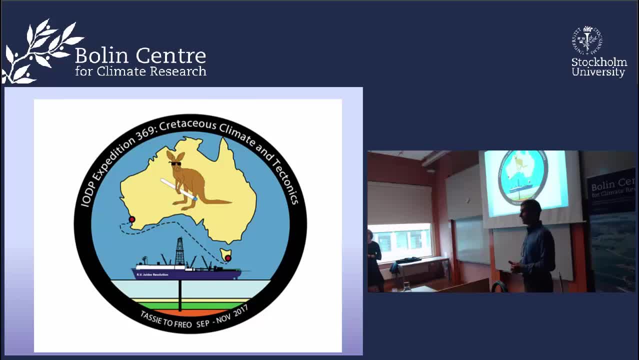 will fit with our fossil and sediment record. So I think we're going to have to see what we can do. If we don't know what's going to happen, we're going to have to do it again. So I think that's a pretty good way to go about it. 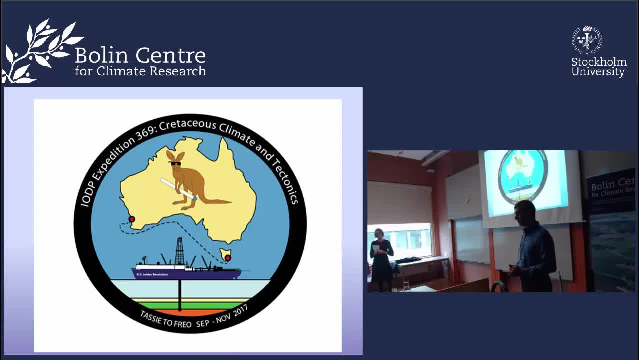 But I think one of the things that's interesting to me is that, from the perspective of the human being, people are being more aware of their own life, their own emotions. They're not going to be concerned about. like well, I'm going to die. 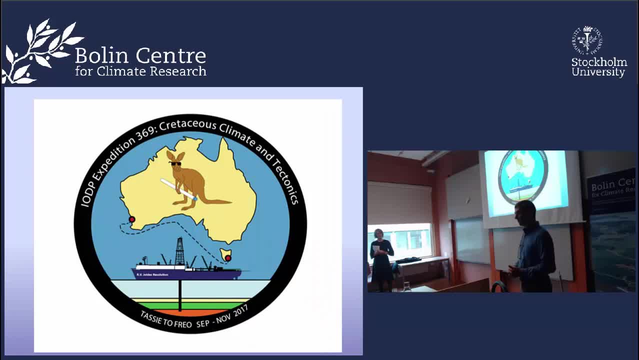 And then there's the human being, And I think that that's going to be a real problem And that's why we're going to have to see what we can do to get that out of the way. You know what I'm saying.